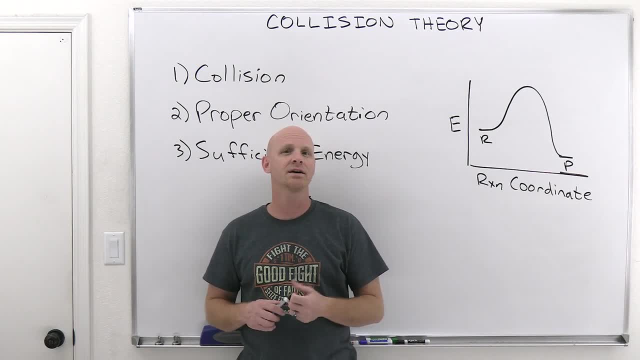 start off with collision theory, and this really gives us kind of a conceptual understanding of the requirements that need to be met at the molecular level for a chemical reaction to take place. And then we'll finish this off with the Arrhenius equation, which is going to show the 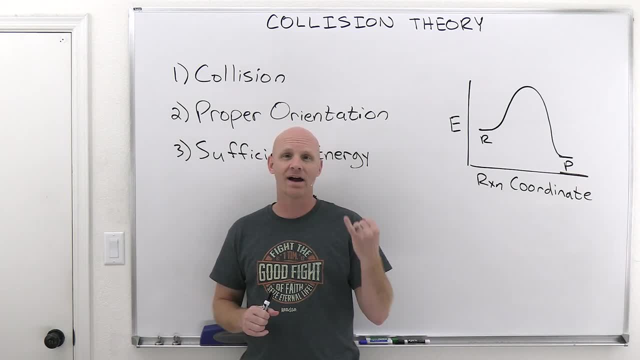 dependence of the rate constant that lowercase k on both the activation energy and the temperature. So we'll kind of get a little bit of a conceptual understanding and put it in kind of a mathematical description, but we're going to have some calculations to go with it as well. So let's 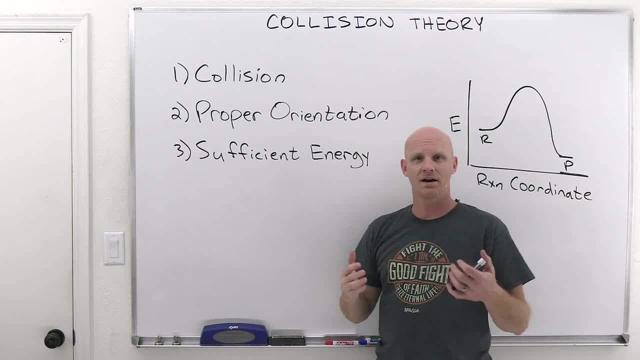 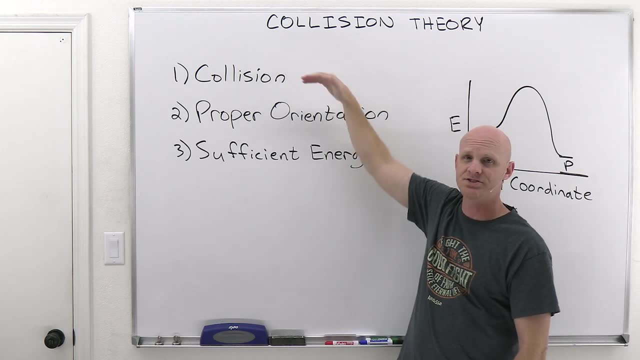 start with collision theory. And again, collision theory is the kind of at the molecular level, the requirements that need to take place for a chemical reaction to occur, And the first of those requirements is there's got to be a collision. So if two molecules are going to be reacting with 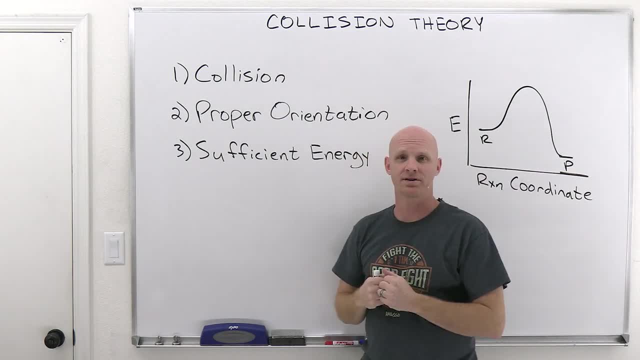 each other, then they need to collide with each other. So that's the first part, And you can kind of see why higher concentrations of reactants generally lead to faster reactions, because if you have more reactants closer together, then they're going to collide more often. 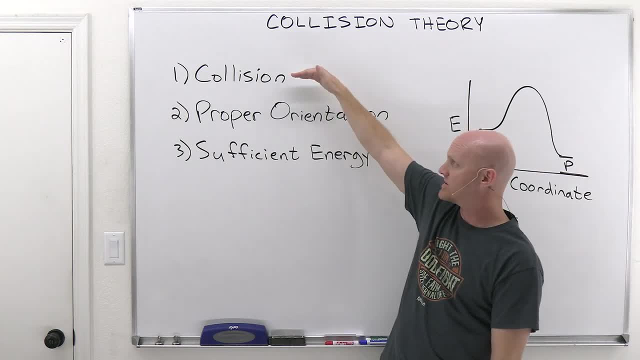 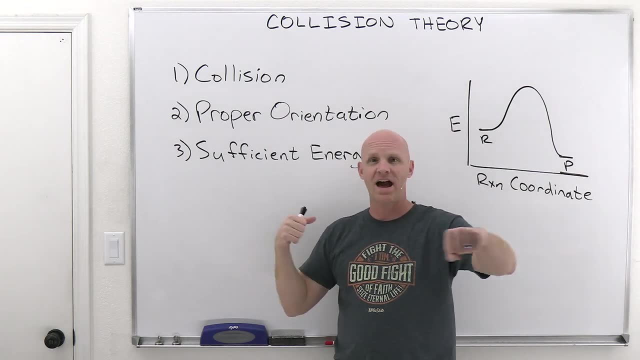 which is going to lead to a faster reaction. But that's not enough. In addition to a collision, the molecules actually have to collide when they have the proper orientation, And so we like to think of that. when this collision happens, that to kind of kickstart this reaction, you're going to have bonds breaking, And so it turns out. 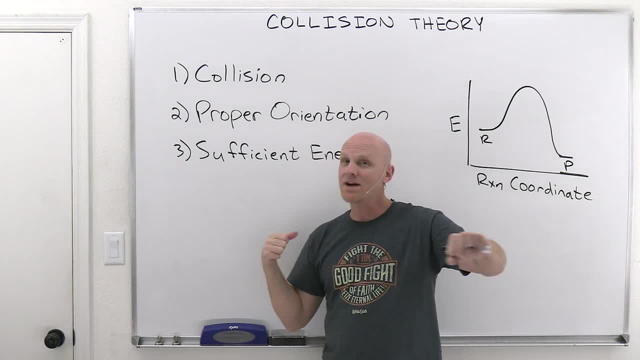 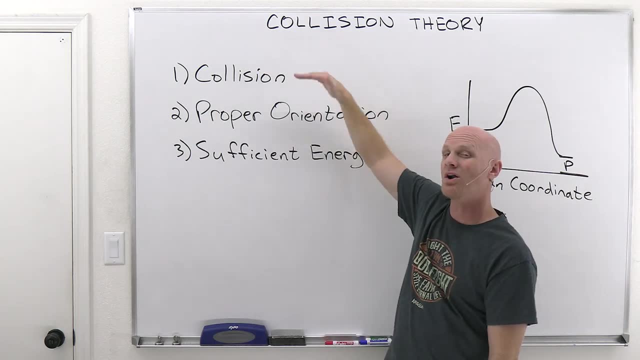 you know, in the parts of the molecule where these bonds are being broken, those are the parts that have to be involved in the collision, or else these molecules just bounce right off each other and no reaction happens, And so again you've got to have a collision, but also the molecules have. 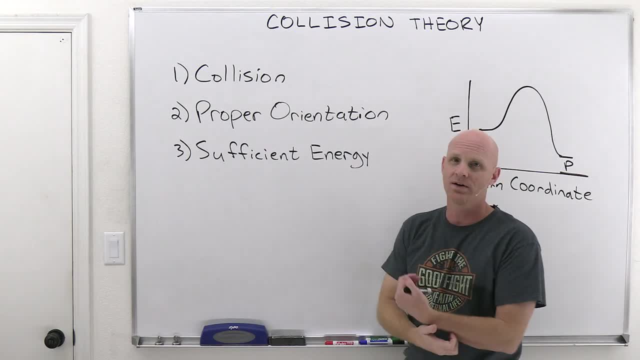 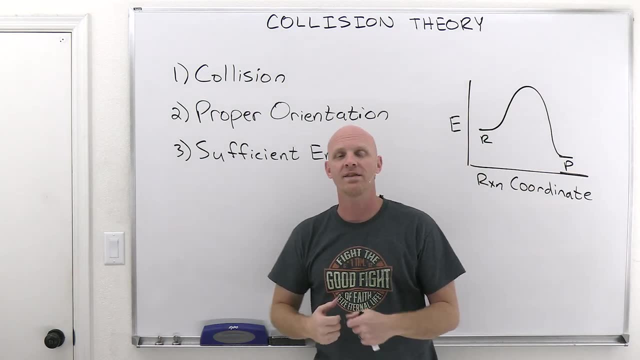 to have the right orientation during that collision as well. But even that's not enough, Turns out. they've got to have sufficient energy during this collision, So they've got to have been moving fast enough when they collide that they can break these bonds, And what this. 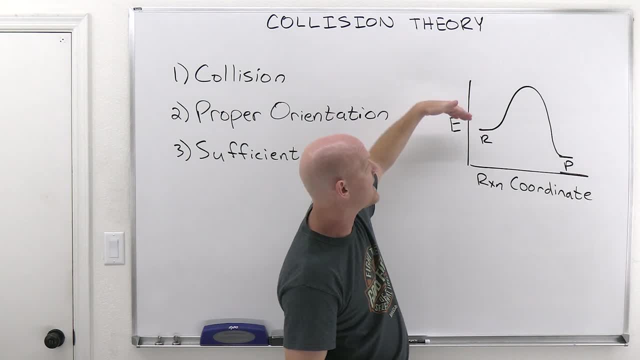 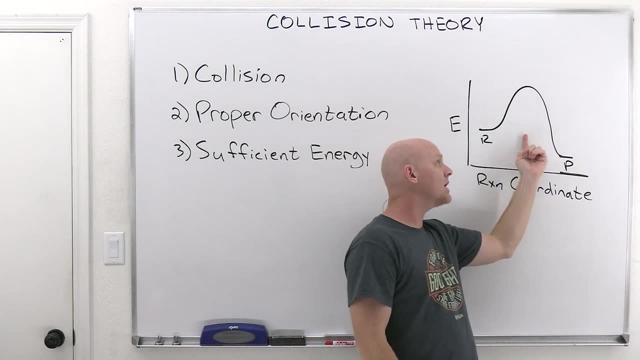 translates into and related to something we talked about in the last lesson, is they've got to have enough energy to get over that activation energy barrier. We often associate the activation energy in a reaction with the bonds that are being broken, And so if two molecules don't have 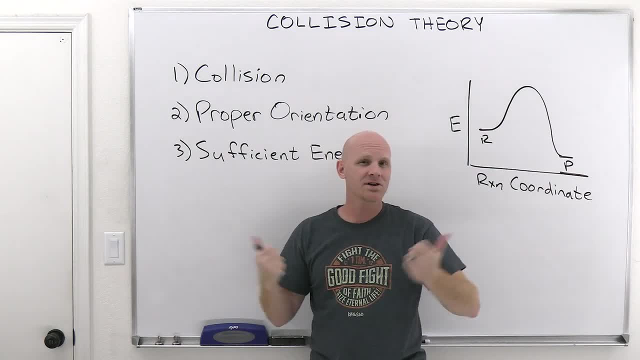 enough kinetic energy going into that collision, then they're just going to bounce off each other again, even if they have the right orientation. So they've got to have enough energy to get over that activation energy barrier. So those are our three requirements. We've got to have a collision. 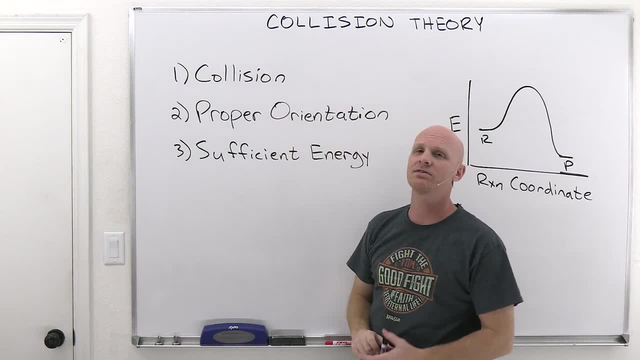 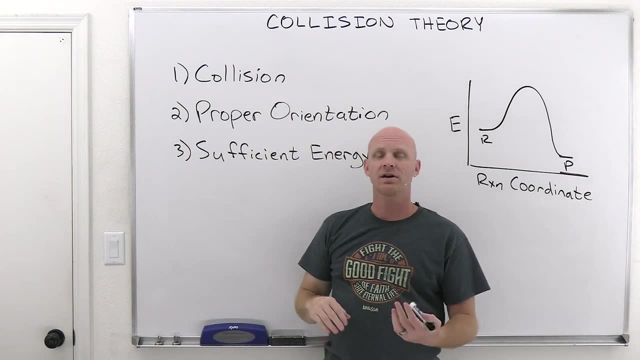 we've got to have the molecules in the right orientation and they have to have enough energy to get over that activation energy barrier. Now you've got to understand these three parts to collision theory, but you're also going to understand how we use this to explain from. 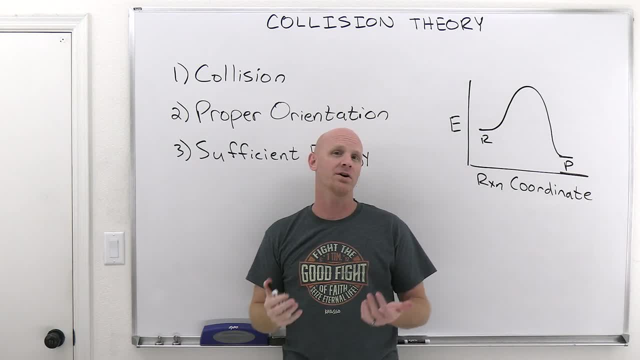 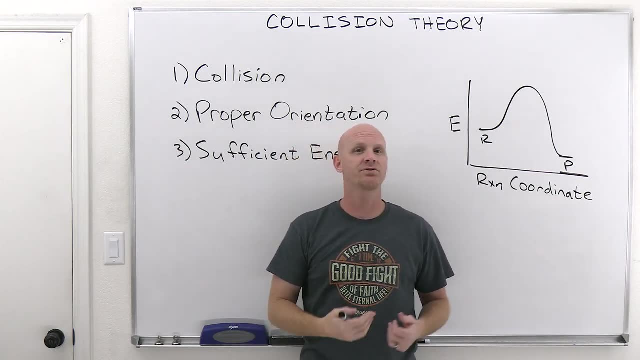 a conceptual level why reactions tend to go faster at higher temperatures And so at higher temperatures. you've got to realize that on average, molecules are moving faster. Their average kinetic energy goes up. Now are all molecules moving faster at higher temperatures? 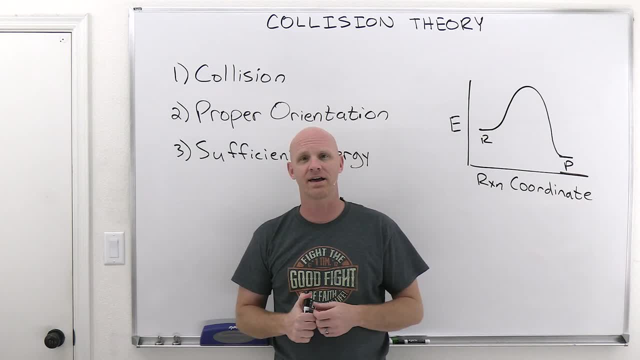 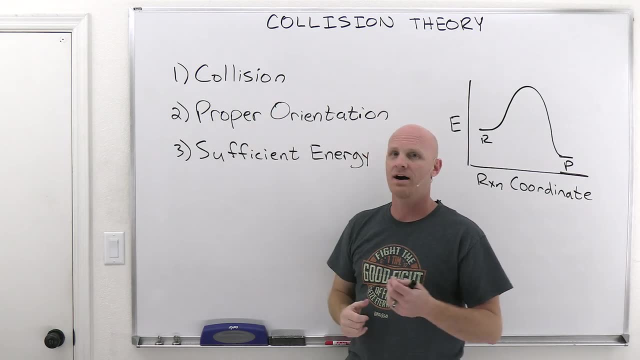 No, but the average shifts towards higher kinetic energy. So what's really going on here is that if you have molecules moving faster, well then they're going to collide more often, And so that's the first place that we're going to see temperature play a role. It's just you get a greater collision. 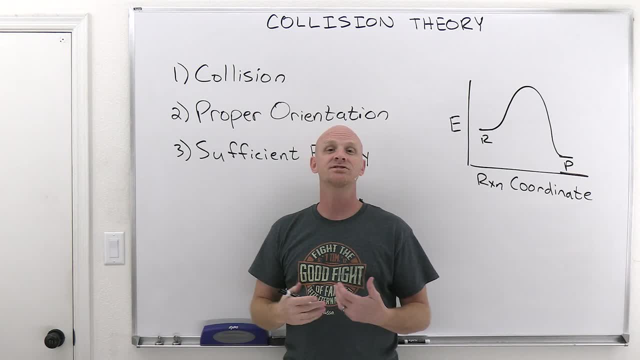 frequency is sometimes how it's worded And that just means that collisions are happening more frequently. And if you have collisions more frequently, then you're going to have more of those collisions more frequently that lead to a chemical reaction. But the other place- temperature. 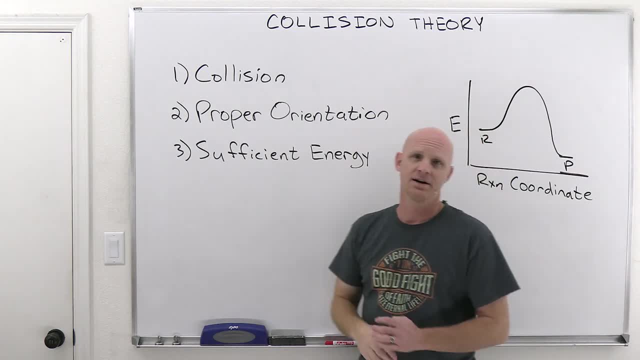 plays a role is in this last part, with sufficient energy. So it turns out you can't change the proper orientation. Only a certain amount of energy can change the proper orientation. So percentage of the collisions are going to have that right orientation and you can't really. 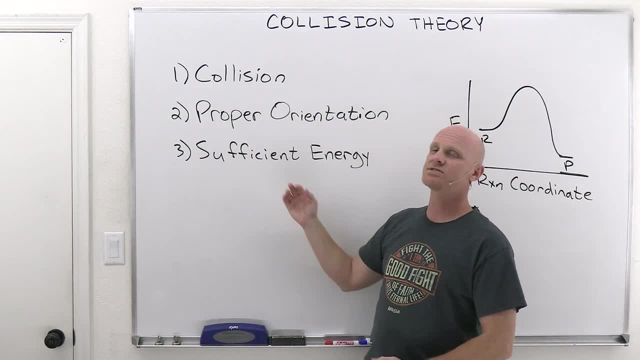 change that by temperature. But what temperature is going to do is it's going to change, It's going to increase the percentage of molecules that have enough energy to get over that activation energy barrier. enough change the percentage of molecule that have sufficient energy. And so the idea is: 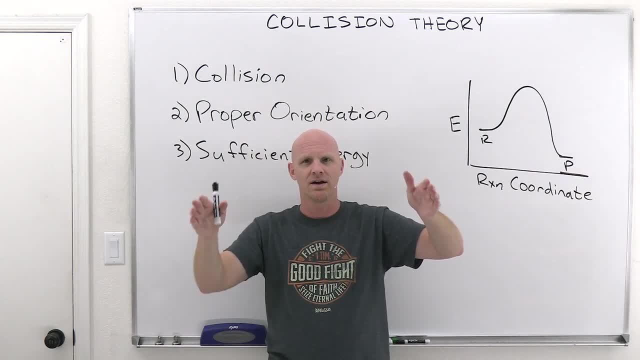 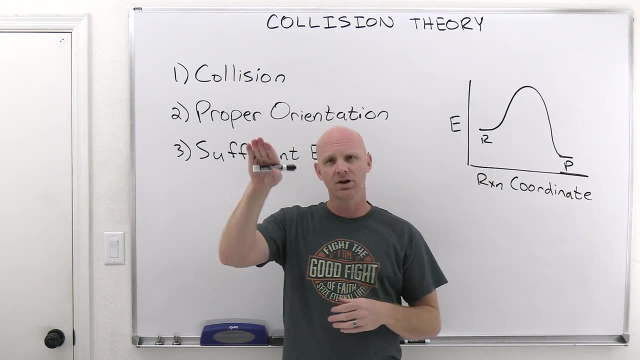 that at any given temperature, you have really this distribution of molecules. So and what you're going to do is shift that distribution to higher energies as you go, to higher temperatures, And so maybe at some low temperature, only 10% of the molecules that have enough energy to get over that. 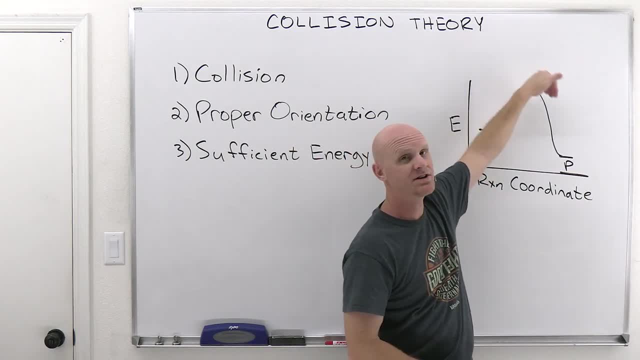 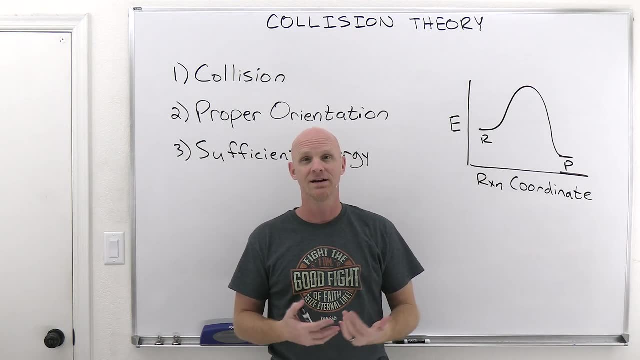 activation energy barrier. But maybe you raise the temperature substantially and now 30% of those molecules actually have enough energy to get over that activation energy when they collide, And so you're going to get a faster reaction as a result, And so that's kind of the twofold effect of 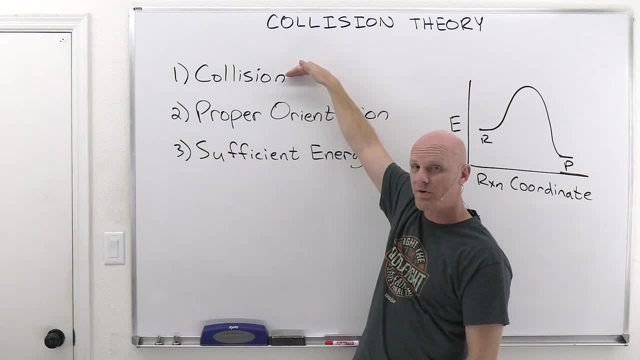 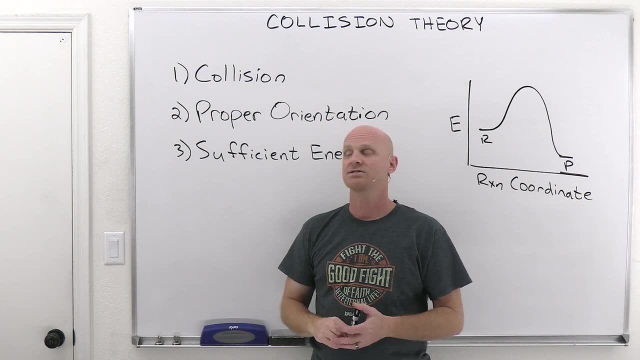 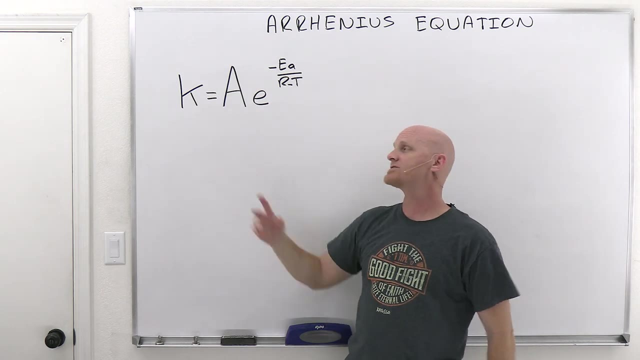 temperature, You get a greater collision frequency, the molecules are colliding more frequently and you get a greater percentage of the molecules having enough energy to get over that activation energy barrier. Now we're going to take a look at the Arrhenius equation here And the Arrhenius equation relates. 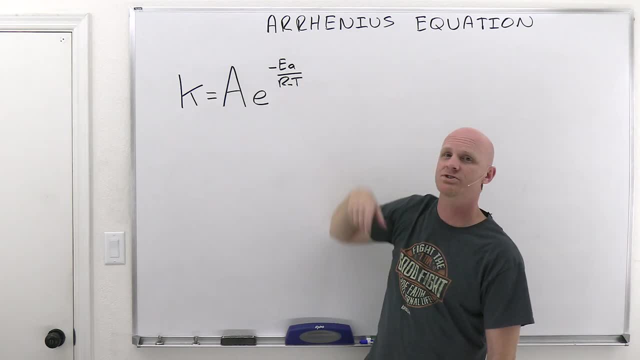 the rate constant to the activation energy and the temperature at which a reaction is carried out. So a couple things you should understand about this lovely rate constant, And so the first part is that this is the same rate constant that showed up in a typical rate law, And so typical rate laws. 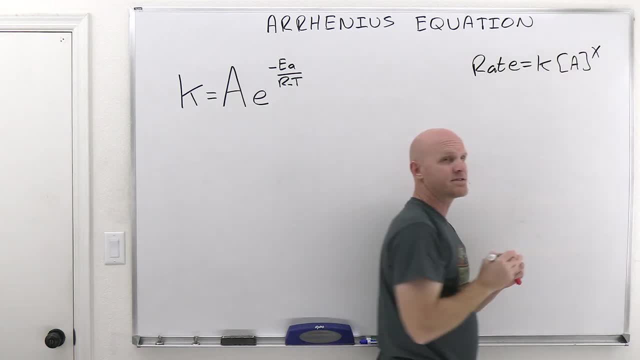 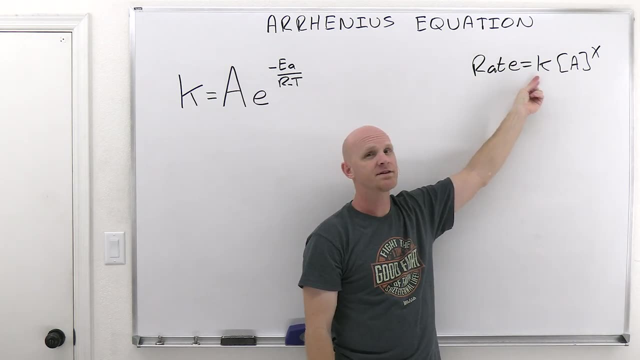 looked something like this: and the rate was directly proportional to the value of the rate constant. So a higher rate constant led to a faster rate and a smaller rate constant led to a slower rate. So that's the first part. you should understand So, but you should also understand the effects of 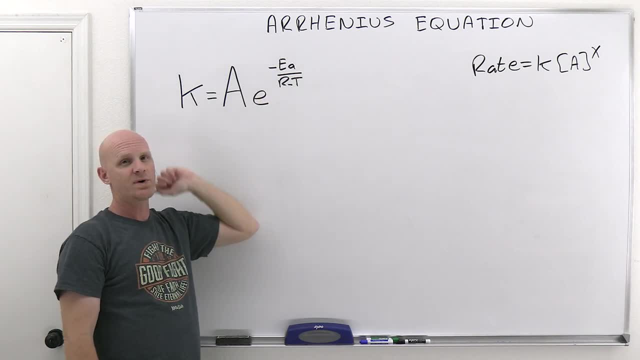 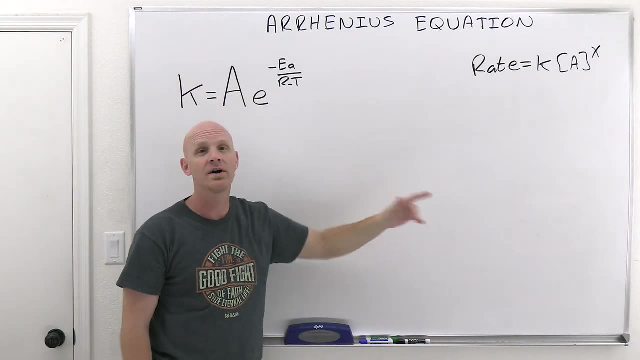 activation and energy and temperature on the value of this rate, constant. Now, in this case, if you understand, oh yeah, you look at this lovely equation and you see a graph that's exponential decay going down. well then, props to you. you are in the vast minority, But you should. 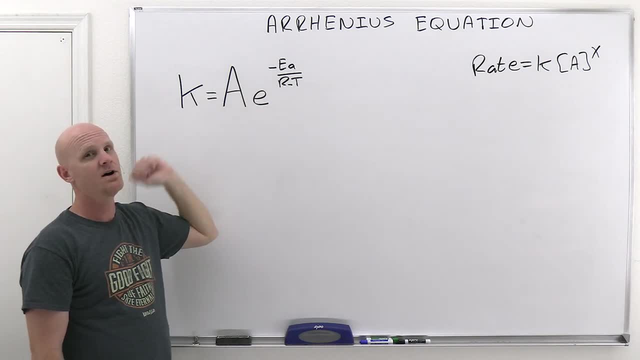 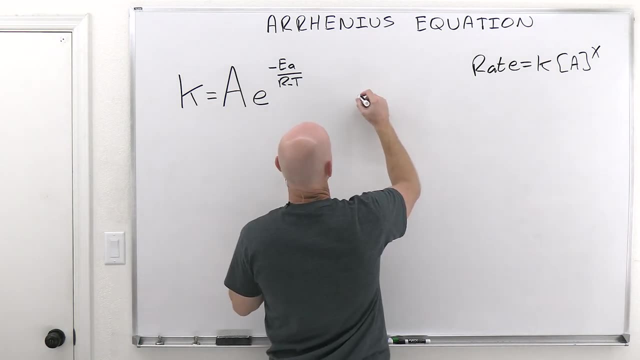 know the impact of both activation energy on the k value and temperature on that k value And, as we just talked about a little bit ago, reactions tend to go faster at higher temperatures And so as they go faster at higher temperatures, it's because you get a higher value of the rate constant. So it 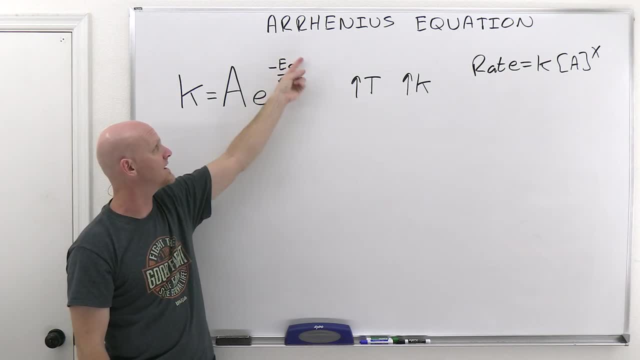 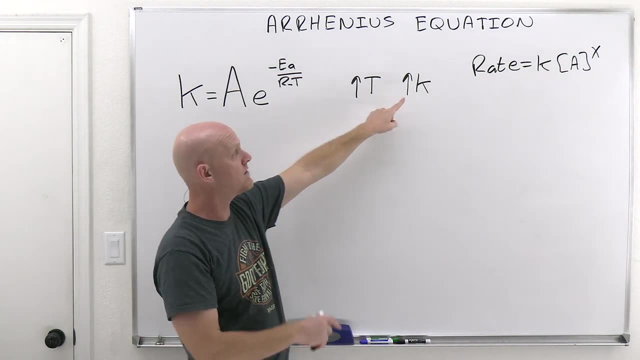 turns out, a larger temperature here means you're going to have a smaller negative number for the exponential, which actually leads to a higher value. Well, again, I don't care if you really understand that mathematically, but you do need to know the result here: that a higher temperature. 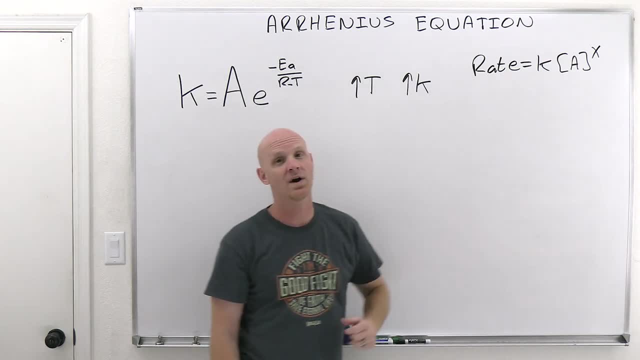 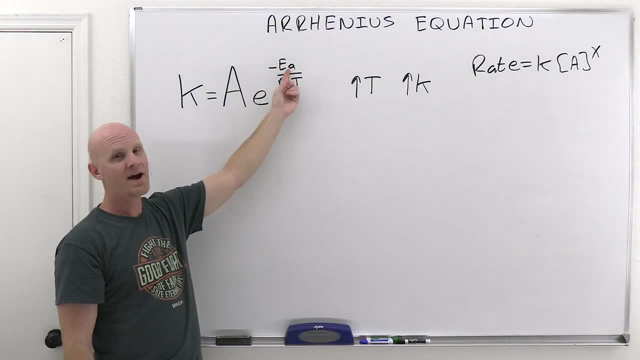 leads to a higher k value, and a higher k value is going to lead to a higher rate. So there's our mathematical influence of temperature on that rate. Now, if we look at the activation energy, it's the exact opposite. A larger activation energy means you have a bigger energetic. 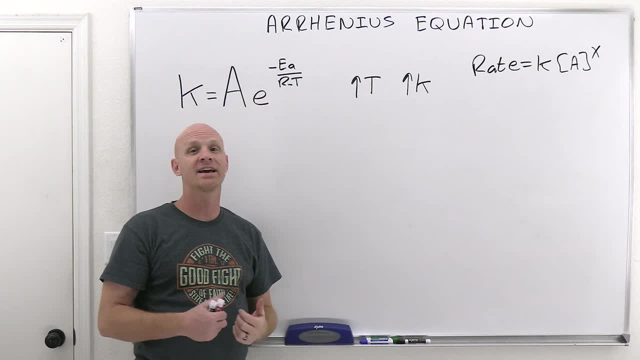 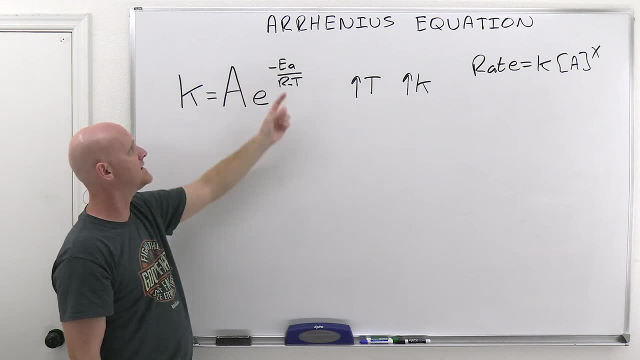 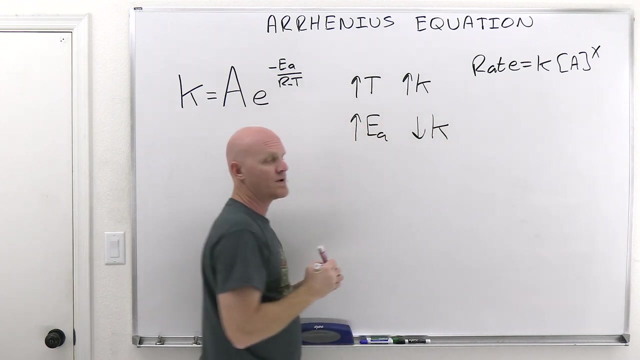 hill to get over, and less molecules have enough energy to get over that hill, And so you're going to have a smaller rate, a lower rate, And so in this case it's actually through the rate constant yet again, And so a larger activation energy is going to lead to a smaller rate constant, And so 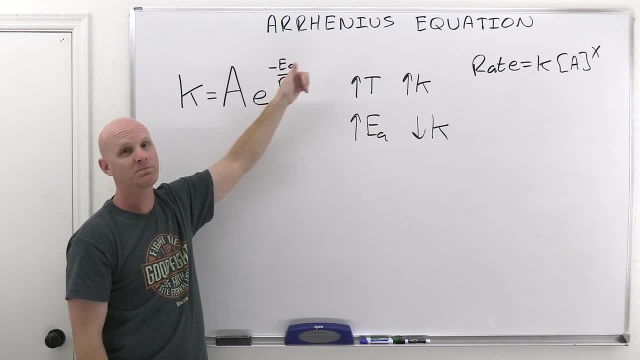 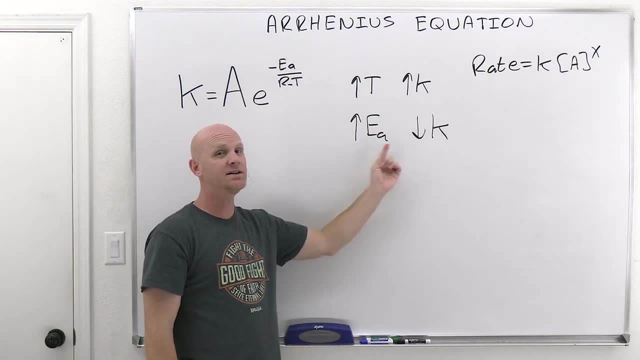 the idea now is that with a larger activation energy, you have a more negative exponential which is going to make your k value go down. And again, if you can't see that mathematically, I don't care, but you definitely need to understand this relationship that a larger 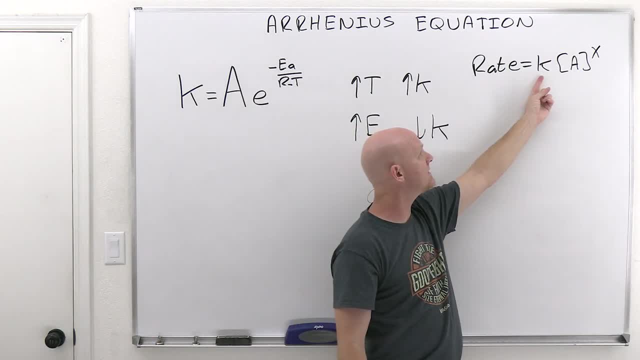 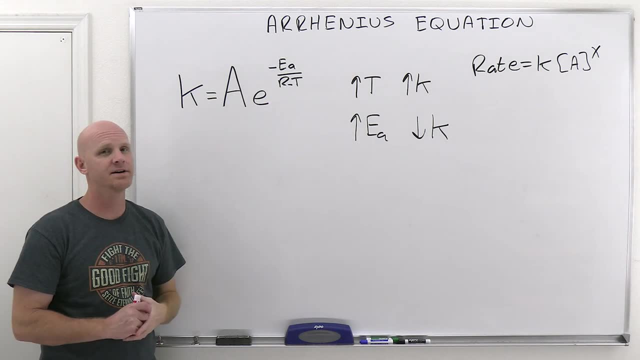 activation energy leads to a smaller rate constant, and that smaller rate constant leads to a slower rate. All right, we take a little closer look at this lovely Arrhenius equation. There's really two parts to this. You've got this first part, So in this first part it's called the Arrhenius. 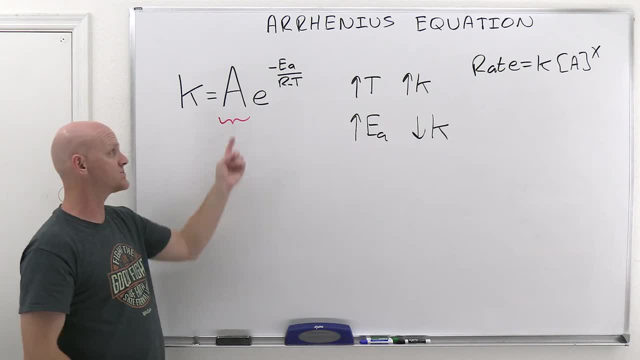 constant, or some people call it the pre-exponential factor, since it's written before the exponential factor. This guy is a constant for a given reaction, But it is related to the proper orientation of the molecules when they collide And there's some different geometrical spatial factors that kind. 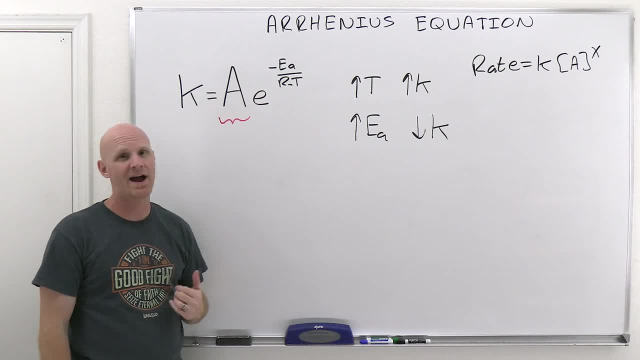 of factor into it. But the big thing I want you to realize, it's constant for a given reaction and it is related to the proper orientation of the molecules, And so you can kind of think of it as the fraction of molecules that actually have the proper orientation when they collide. 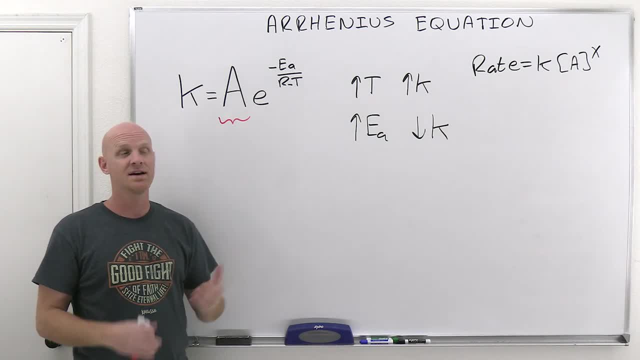 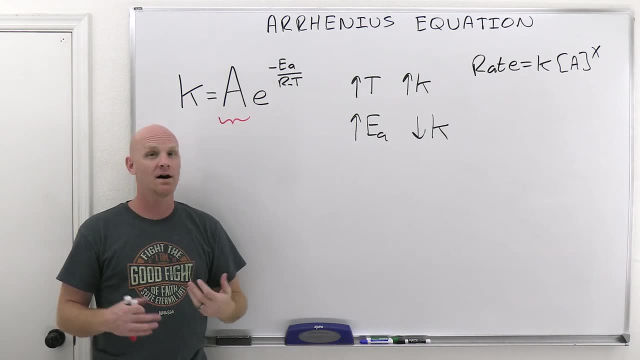 And so if, for a given reaction, only 10% of the collisions have the right orientation, well then this would be 0.1.. That's kind of how it works And you can't really change it for that reaction under that particular mechanism. Now, the other part here is this exponential term. 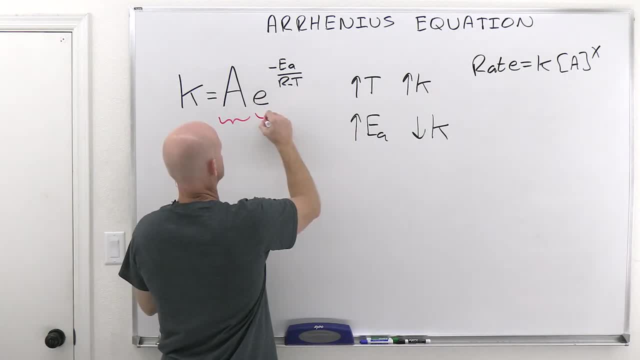 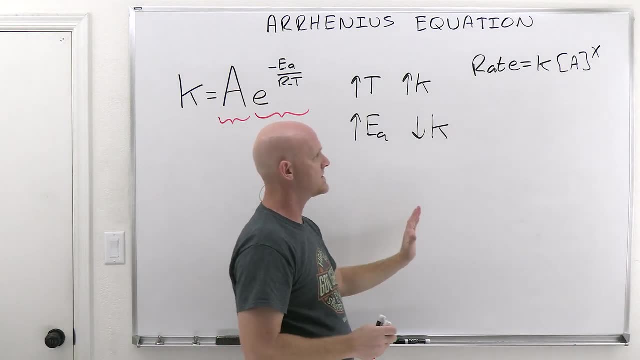 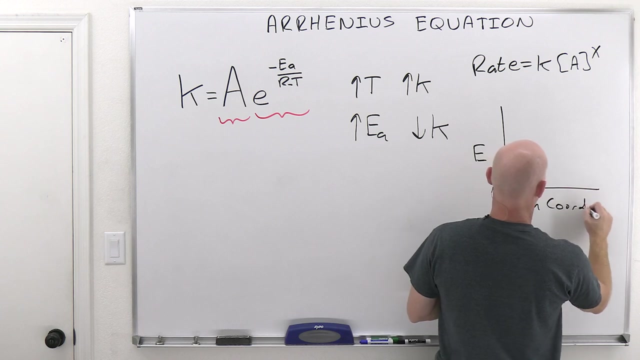 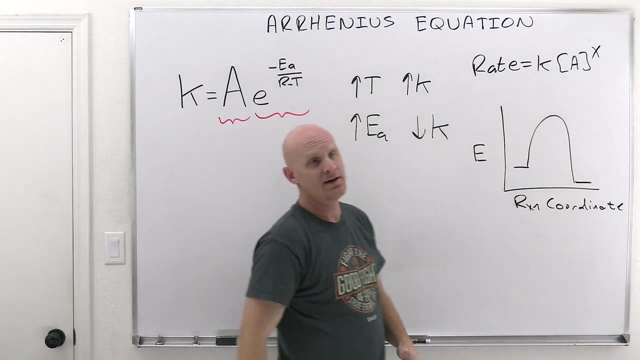 And this exponential term is really the fraction of molecules that have enough energy to get over that activation energy barrier. So we saw earlier we looked at our reaction coordinate diagrams So that we had an energy hill to kind of get over And the idea here is that this is the 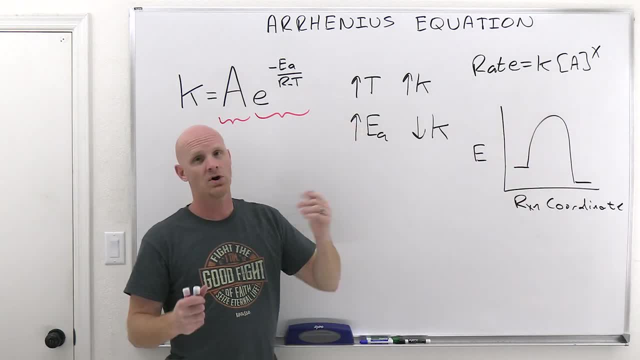 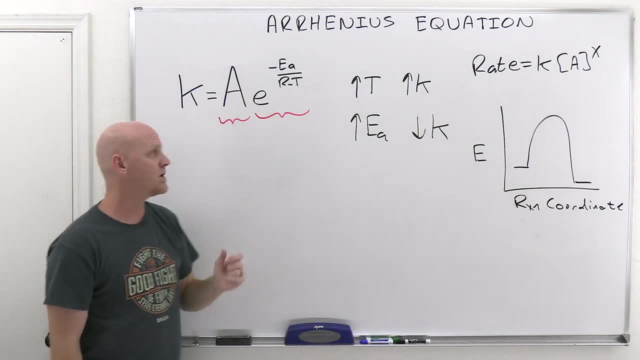 fraction of molecules that actually have enough energy to get over it. And so, if you know, at a given temperature only 20% of the molecules have enough energy to get over that hill. great, we factor that in right here And over here. if only 10% of the molecules are in the proper 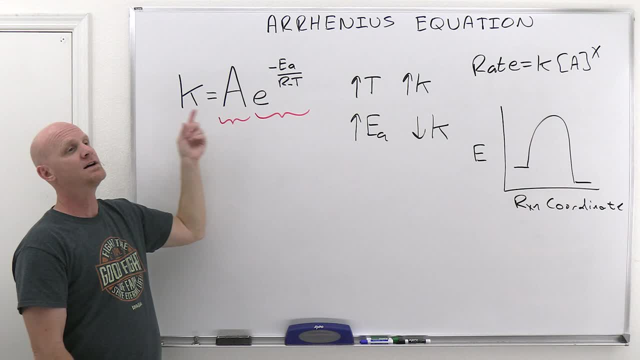 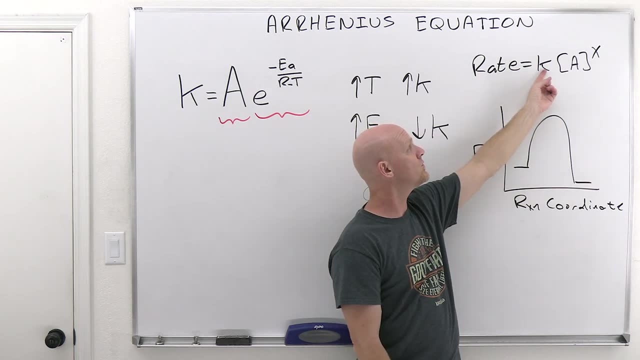 orientation that gets factored in right here, And both of those combined give us effectively the rate constant, And so the rate is dependent upon the concentrations of the molecules that are reactants, but also on this rate constant, which factors in again your proper orientation and 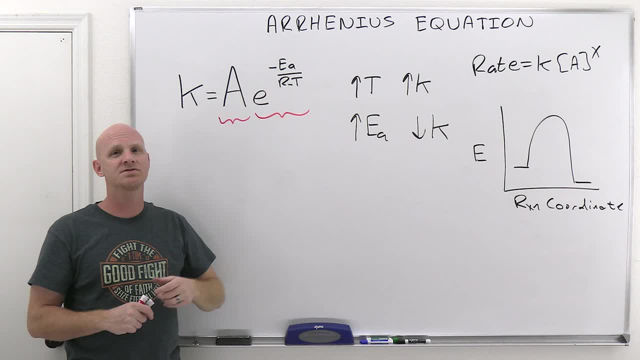 sufficient energy, And so all of this kind of relates back to that collision theory. With higher concentrations you get more collisions, So and then this describes the proper orientation and this guy the fraction of molecules with sufficient energy. So that's where that's kind of coming from. 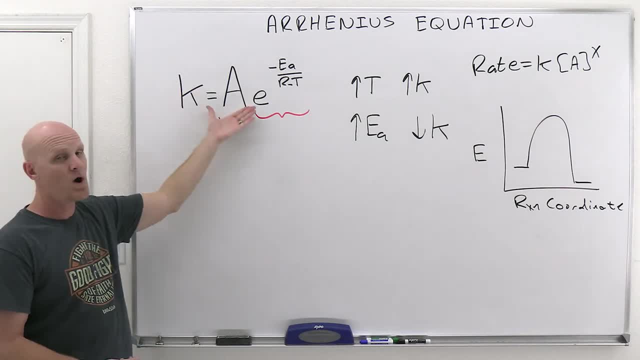 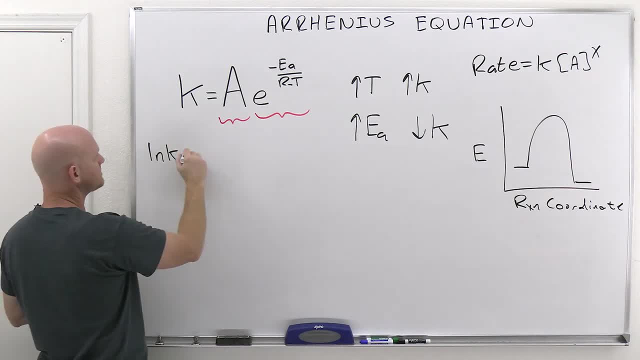 the natural log of this you're going to get, ln of k is equal to: and if we take the ln here, it's really the product of two terms here, And when you've got logs of a product, you can actually split it out into separate log terms And so we've got the sum of two separate log terms like this. 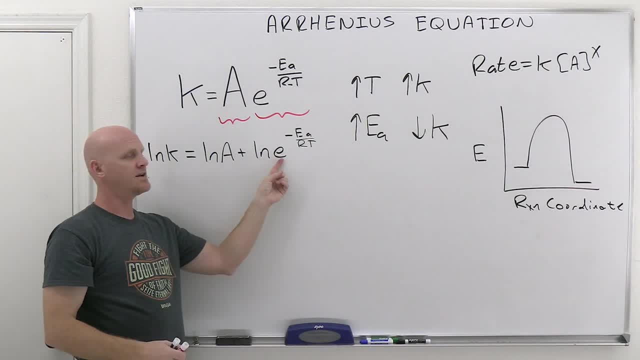 and I'm going to change the order here. But it turns out that natural log and exponential are inverse functions. they cancel each other out, And all you're left with is simply just negative Ea over Rt, And then this one's just going to be ln of a. Now I'm going to change the order here. I'm going to do. 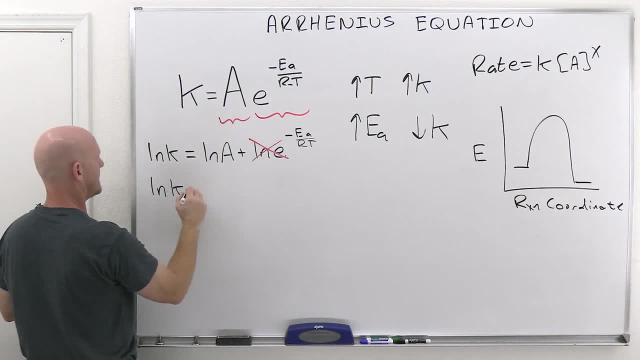 that for a reason, I'm going to rewrite this equation as ln of k equals negative Ea And instead of writing Rt all together, I'm actually going to separate this out into one over t. But this essentially, is just negative Ea over Rt, and then plus ln of a Cool, And that's the way it'll. 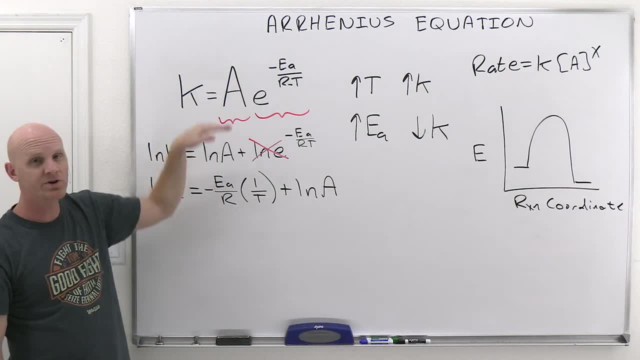 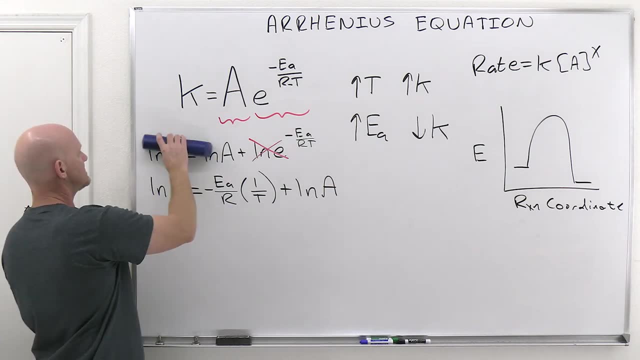 commonly be presented, So most of the time, students are going to be provided with both versions here of the Arrhenius equation. It's not something we often have students memorize. I apologize if you're one of those that has to memorize it. So that's the form it's going to be. 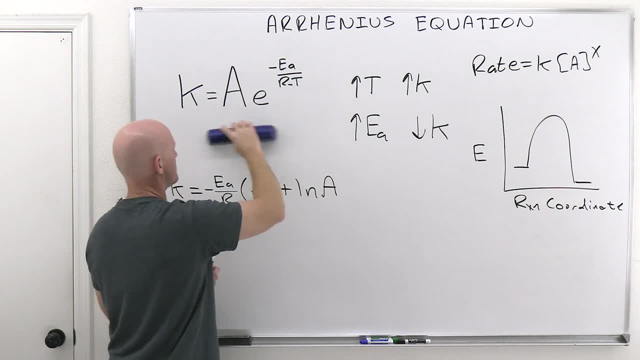 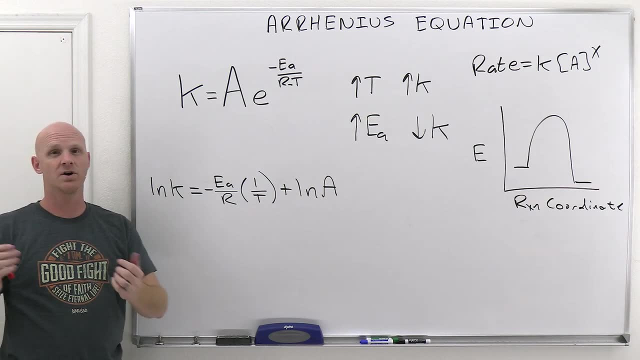 often given in, And we do that for a reason, So oftentimes we can now get a linear graph out of this that helps us actually solve these things, you know, like we do in an experiment in the lab, both to get the Arrhenius constant as well as to solve for the activation energy. 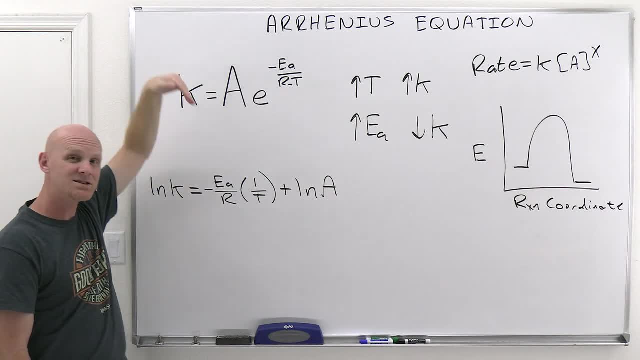 So this top graph here, this is not a linear graph, It's an exponential and you get exponential energy. But for this bottom one, here if you graph the right things you can get a straight line, And the idea is that we're going to kind of match this up to the slope intercept equation of a line. 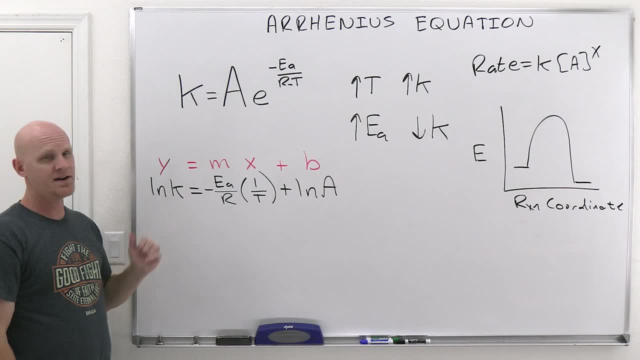 y equals mx plus b, And so as long as I plot the natural log of k- not just plain k, but the natural log of k on the y-axis, and then 1 over temperature in Kelvin on the x-axis, I will get a straight. 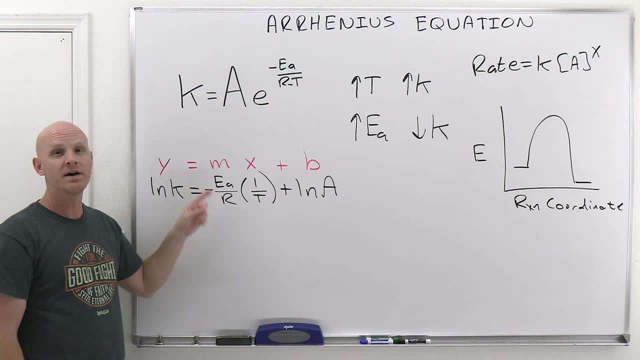 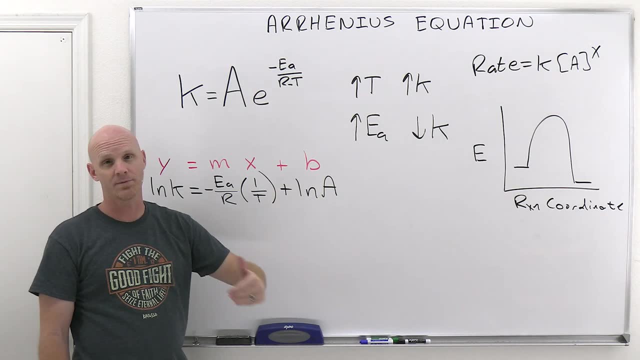 line And the slope of that line is going to equal the negative activation energy over R, And from that slope I can determine the activation energy. And then the y-intercept here is going to equal the Arrhenius constant and I can determine the Arrhenius constant from that. Now much more. 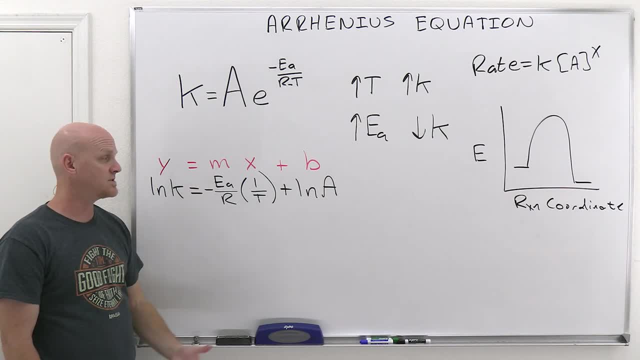 commonly in gen chem, we're going to have students actually determine the activation energy, But in principle, again, you could totally determine the Arrhenius constant And sometimes in some of the lab work we have you do, we'll have you get both And we'll have you, you know, run a reaction at a. 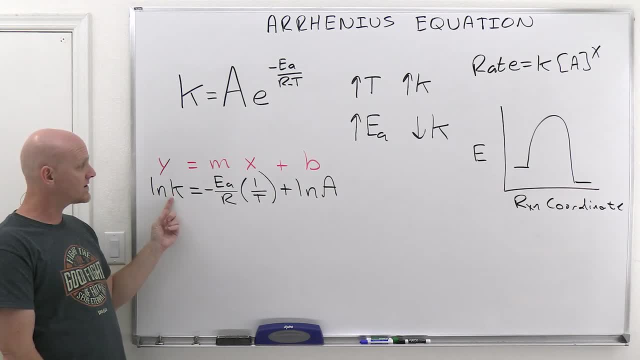 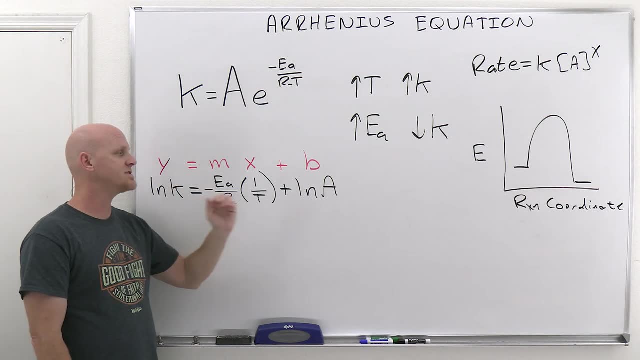 bunch of different temperatures and get different values for the Arrhenius- I'm sorry for the rate- constant at different temperatures, And then we'll have you plot ln of k versus 1 over t and use the slope to get the activation energy and that y-intercept. 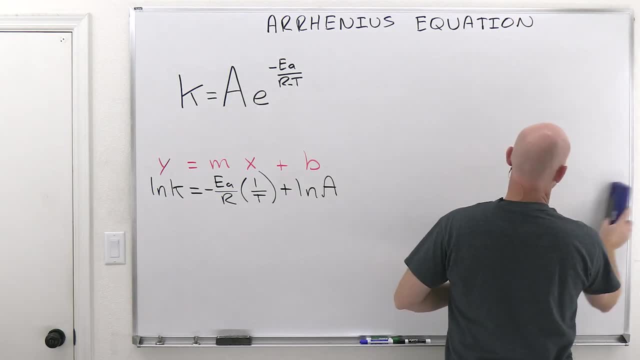 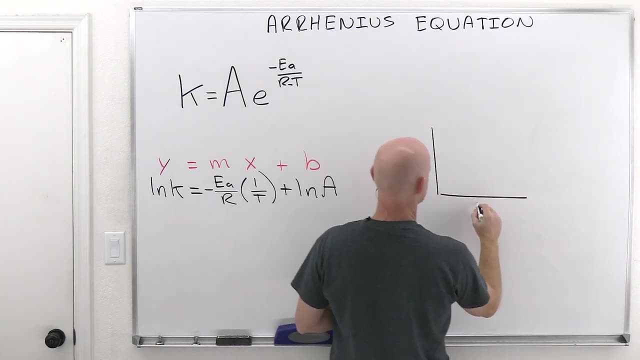 To get the Arrhenius constant. Let's take a look at this graph real quick Again. ln of k on the y-axis 1 over temperature, and you got to make sure that's in Kelvin- super important So- and you're going to get a graph with a negative slope. 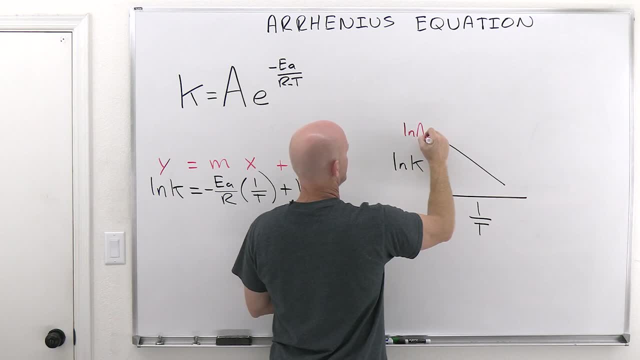 And in this case this point right here is going to equal ln of a and you can get your Arrhenius constant from it. And then the slope on this graph m is going to equal negative slope, Negative ea over r, And so routinely we'll give students a question on an exam in this section. 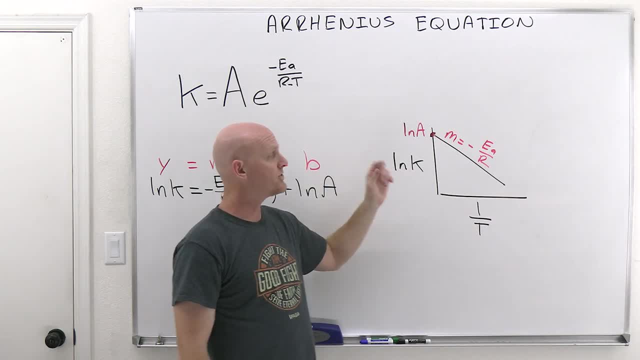 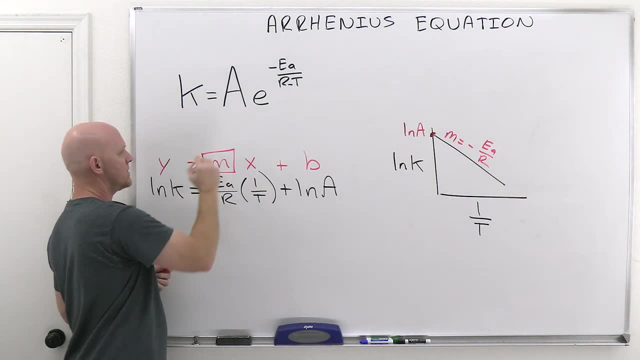 and we'll give you a graph like this: So, and then we'll either give you the equation of the line So, and if we give you the equation of the line, this would be the part to really focus on- what's the numerical value for that slope- Or we'll just say the slope is and give you the slope directly. 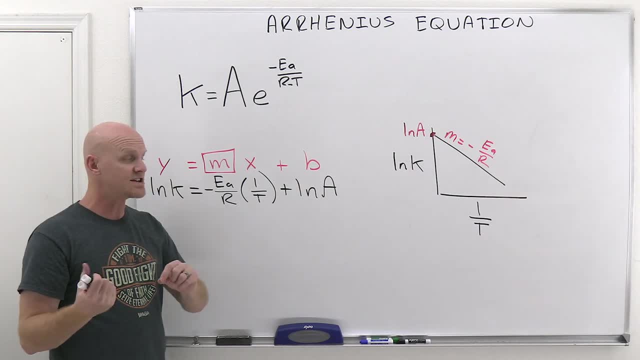 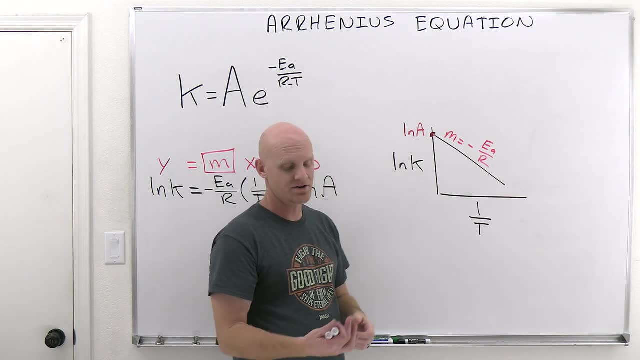 So, but whether we give you the equation of the line or just give you the slope, specifically, it's that slope that you really want, Because you're going to set that slope equal to negative ea over r and then rearrange it to solve for that activation energy, And so whatever numerical value, 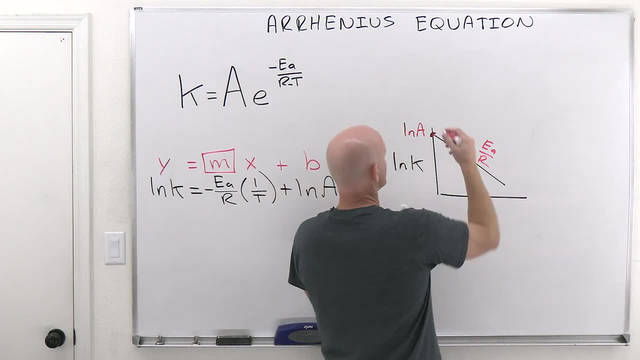 this is. you're just going to plug it in, But if you rearrange that, you're actually going to get that, the activation energy. So we're going to multiply the other side by r and bring the negative sign over as well. It's going to equal negative slope times, r, And that's how you get your. 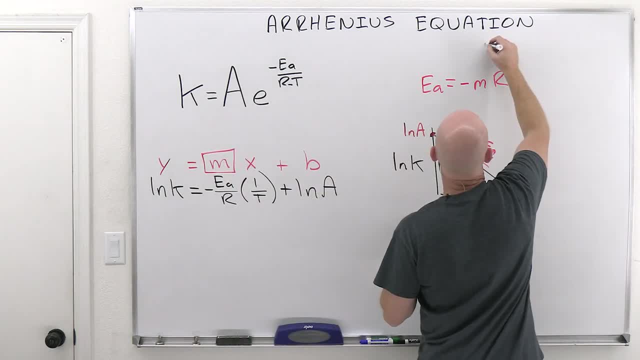 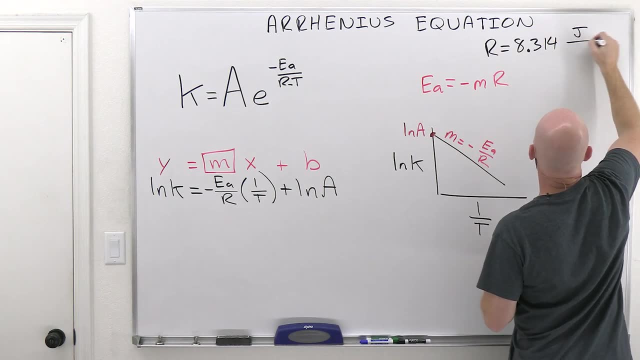 activation energy. Now, one thing you should know here, super important is the value of r, That's your universal gas constant, And we often give students this in a class. So if you're going to do a couple of different sets of units, and when dealing with energy you're most commonly going to 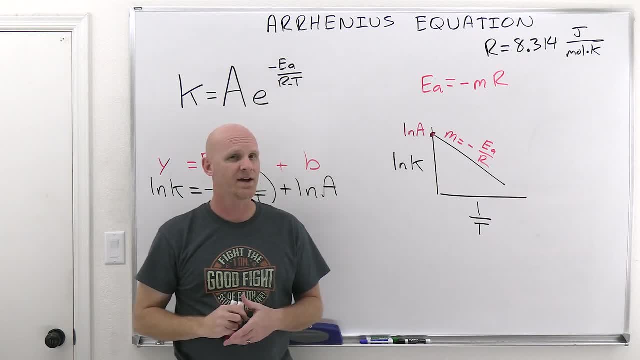 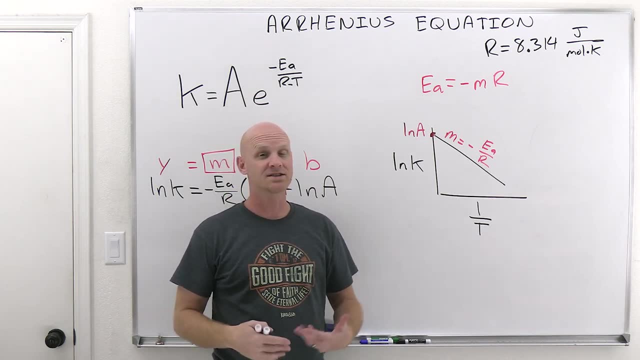 see it given as 8.314 joules per mole kelvin, Whereas when you're dealing with like gases, like in the ideal gas chapter, you're more commonly going to see it presented as 0.08206 liter atmospheres per mole kelvin instead. So, but in dealing with equations involving energy, 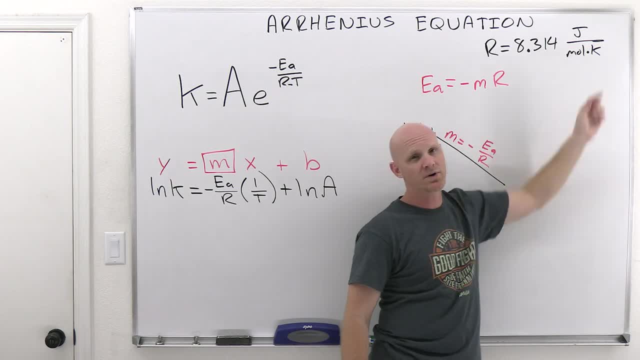 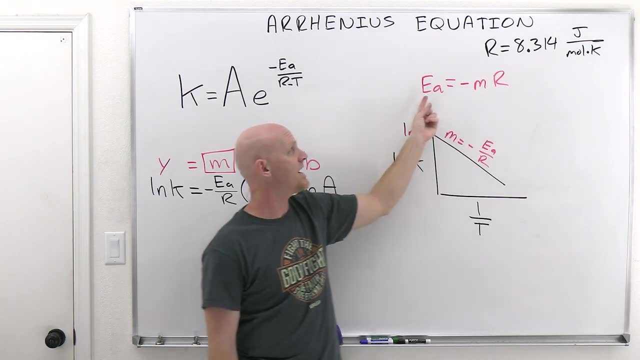 it's much more common to use the SI unit for energy, the joule per mole kelvin, instead. But that being the case, then if you use that value of r here, which is often provided for students, then your activation energy is going to come out in units of. 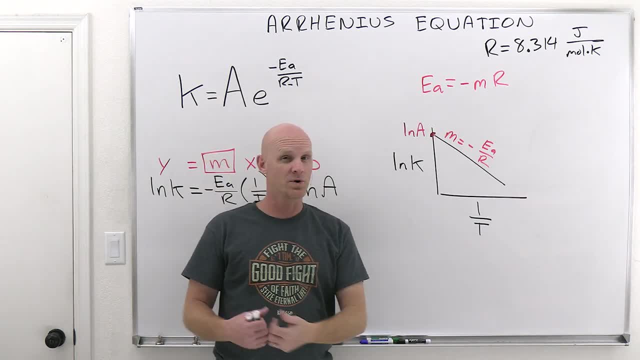 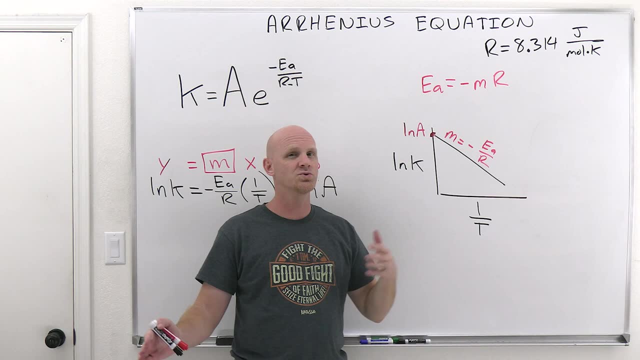 joules per mole, But it's most commonly either provided for you in kilojoules per mole or asked of you on an exam as an answer choice in kilojoules per mole. So you may have to convert it And again to go from joules to kilojoules. you'd end up dividing by a thousand, So just keep that in. 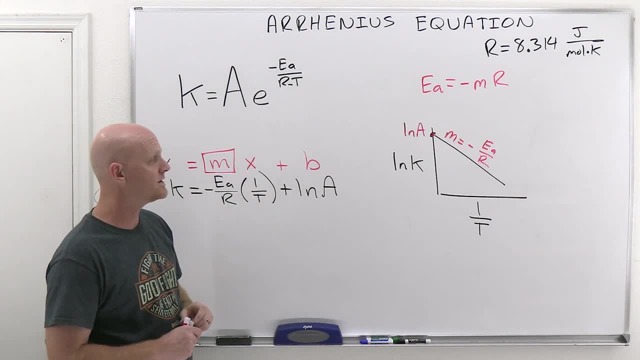 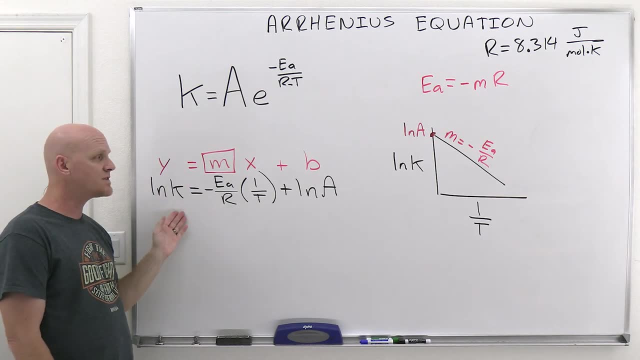 mind, Super important on units here. That'll become important in one other place, as we'll see. So here's the Arrhenius equation. Here's another version of the Arrhenius equation. It's this one that allows us to kind of see the difference between the two. So if you're dealing with 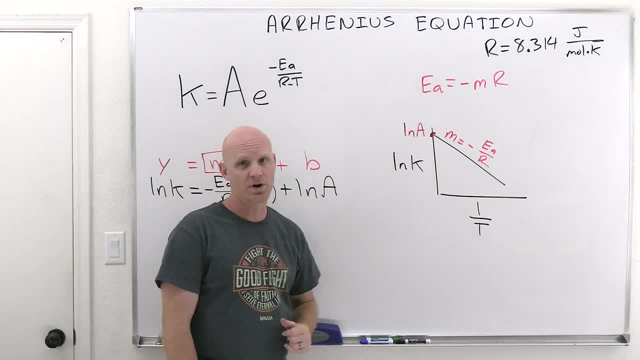 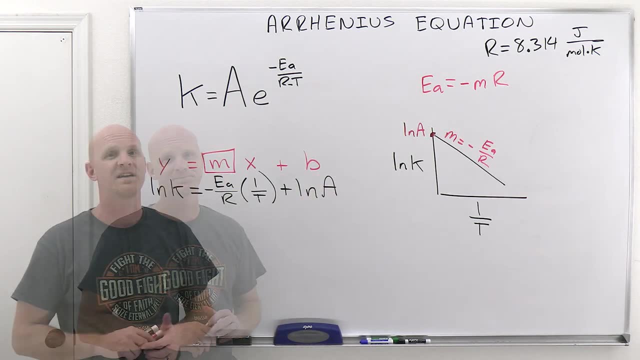 the relationship being linear between L and K and one over T, and how we could use that to solve for the activation energy, for sure, but maybe even that Arrhenius constant. Now there's one other version of this equation So that you might be given- usually not something you have to memorize- 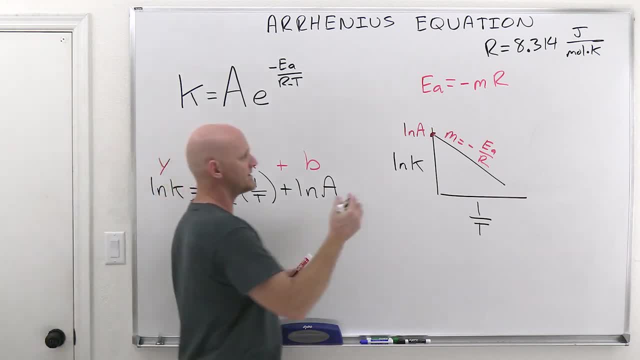 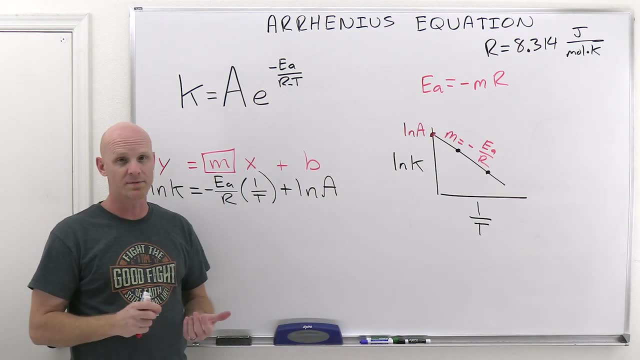 but it's one other version of this equation And essentially it's kind of looking. if you kind of look at where it comes from, you could kind of look at it as connecting two points on that line and calculating the slope between them, And you might recall that slope is rise over run. 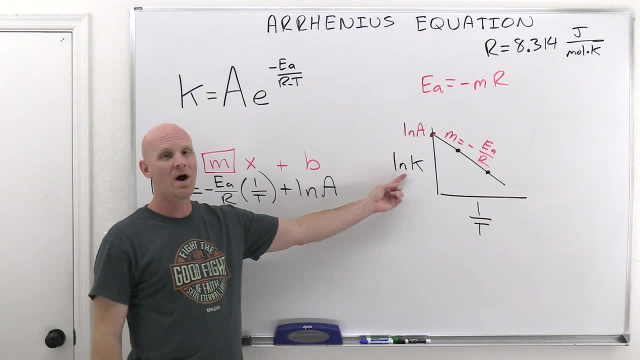 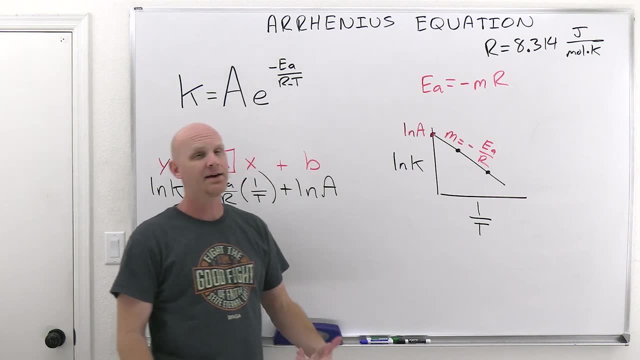 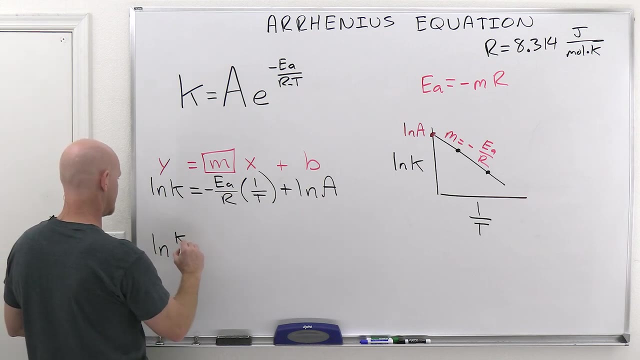 or change in Y over change in X. And well, change in Y would be Ln of K and change in X, in this case, would be the change in one over T, And, ultimately, that's where this next version of the equation comes from. And so this has a few different forms it might take, but I'm going to give you. 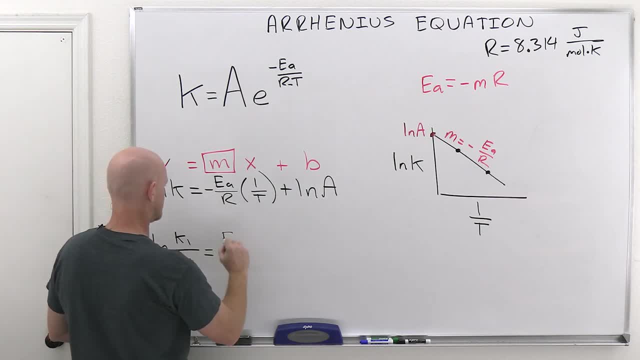 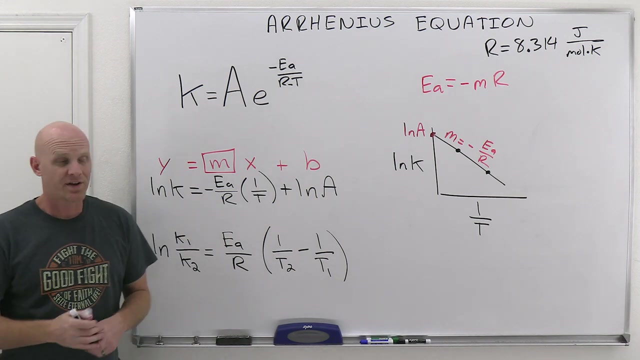 this one. Ln of K1 over K2 equals Ea over R times one over, and in this case I gave it T as T2, minus one over T1.. Cool, Now, this is tricky, So, but you might look at this as kind of being. 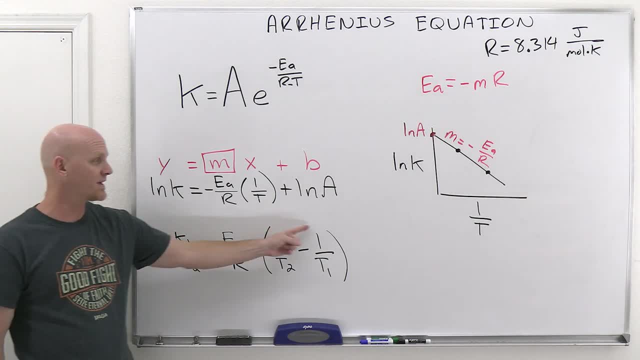 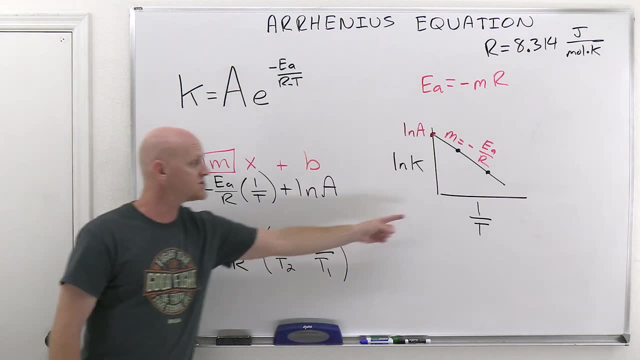 related to delta Y in rise over run, and this being related to delta X. So this is like the change in LnK And you might be like, well, that doesn't look like much of a change. Now this might look like the change in one over T, the change being like final minus initial, So one over T2. 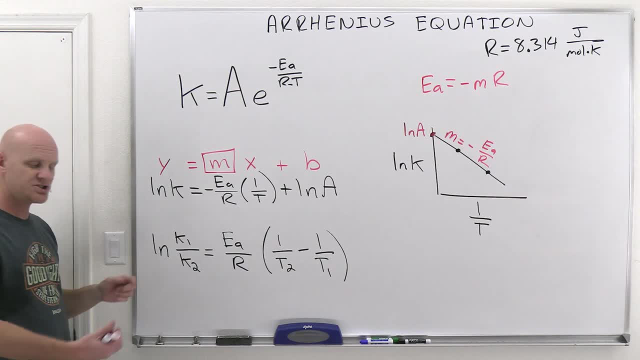 minus one over T1. That makes sense, But this doesn't look like much of a change until you realize that this is the same thing. So this is the same thing. So this is the same thing. So this is written as Ln of K1 minus Ln of K2.. And a property of logs is when you subtract separate. 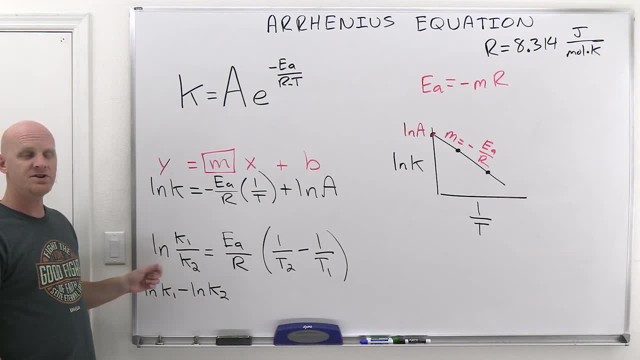 log terms. you can combine them into one log term with division, And so this is the same thing as Ln of K1 over K2.. You might also realize too, that Ln of K1 minus Ln of K2 is exactly the. 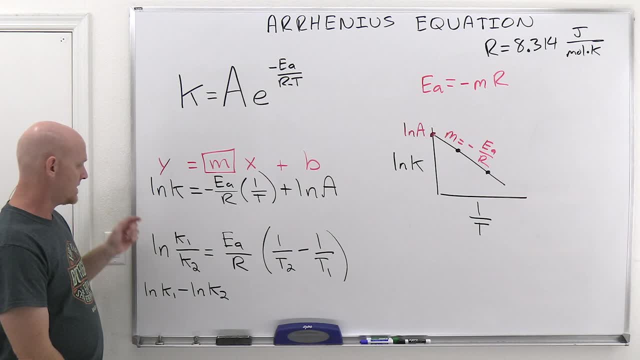 negative of Ln of K2 minus Ln of K1. And so Ln of K1 over K2 is the exact negative of Ln of K2 over K1. And you might be like, well, Chad, I remember the slope was not actually equal to Ea over R, but negative Ea over R And well. 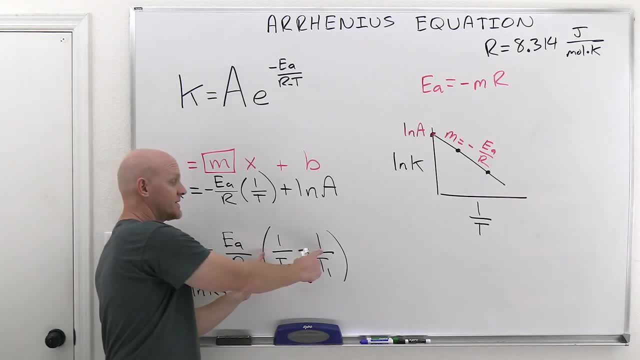 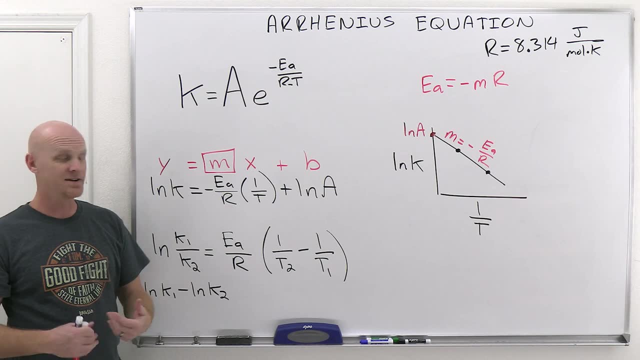 I could factor in that negative sign by flipping these over. I could factor in that negative sign by flipping these around as well. And so there are a few different versions of this equation, depending on what you do with that negative sign, and either leaving it into the equation right here. 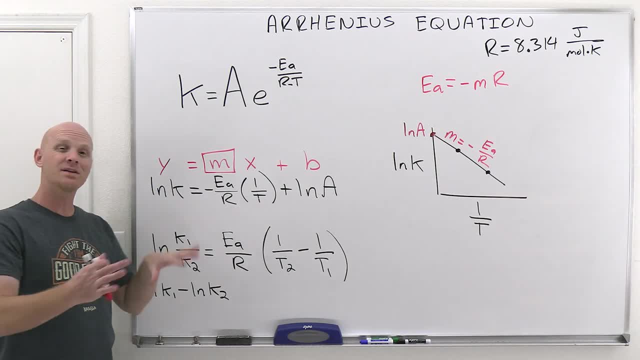 or implementing it in one of these two places. So my apologies, I'm giving you just one version of this equation. They're all a little bit related. Use whichever one you're given, but you do need to be careful. And the big thing is that K1 is the rate constant. 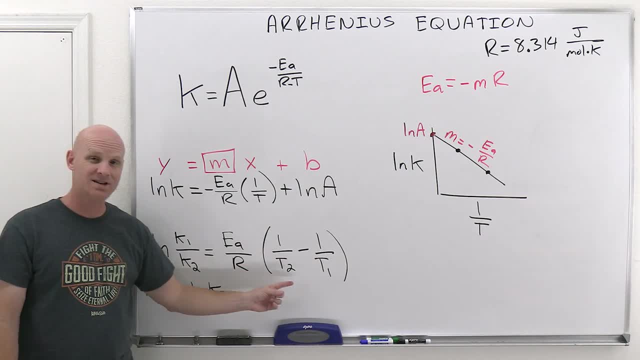 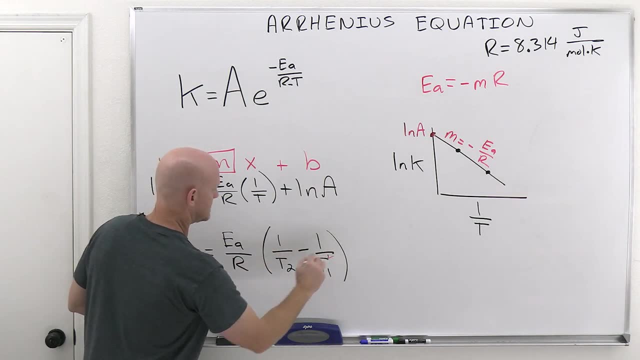 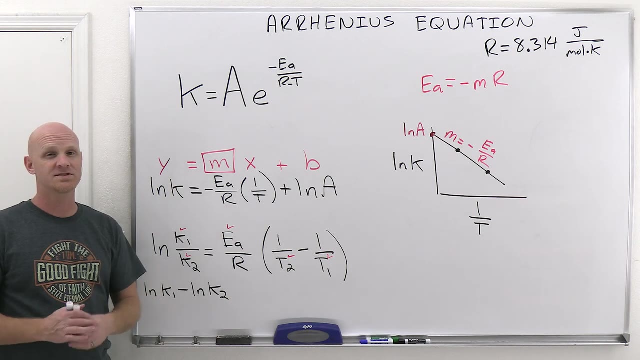 At temperature 1 and K2 is the rate constant at temperature 2.. There are five variables in this equation. There is K1, K2, T1, T2, and the activation energy R is a constant. And with five variables in this equation, it is really common for us to give you four of them and then. 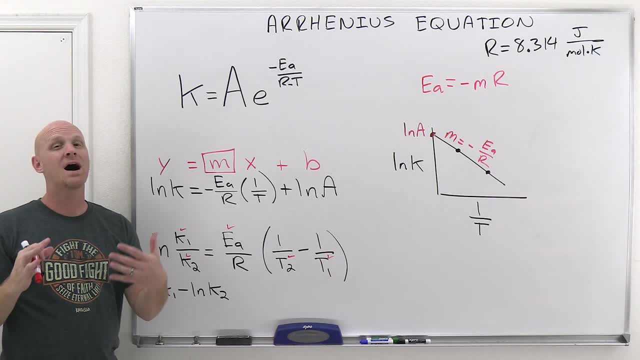 say, solve for the fifth, And if you get this question in your exam, my apologies. It is a pain in the butt. There are several places for you to go wrong here. We're going to do an example calculation, But, upfront, what you need to know is that T1 and T2 have to have to have to be in. 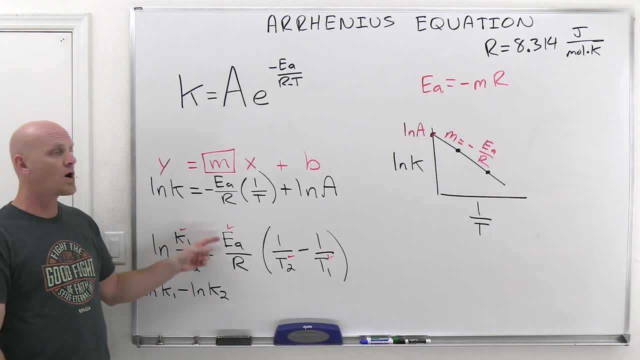 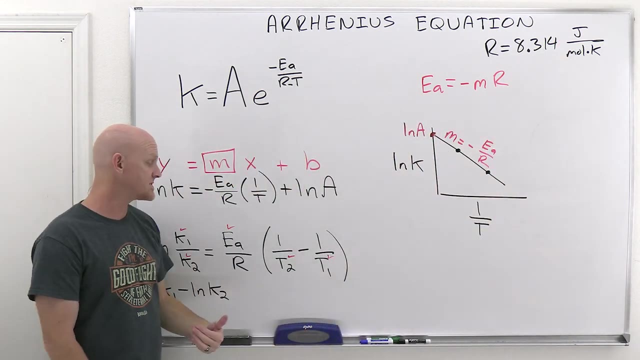 Kelvin, No ifs, ands or buts. And then activation energy and R have to have their units of energy match. Activation energies are often provided to you in kilojoules per mole, but R is often given to you in units of joules per mole. Kelvin. Either make them both joules or both kilojoules, because 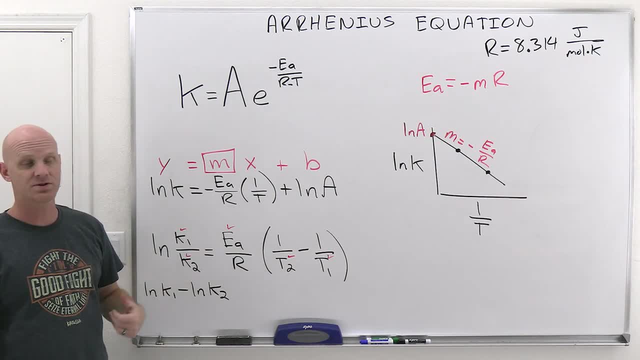 those joules or kilojoules need to cancel when you're doing the calculation here. So those units are the most common places to make errors, besides just plain old algebra and calculator errors. So let's look at an example here. All right, The question we're going to work out here. 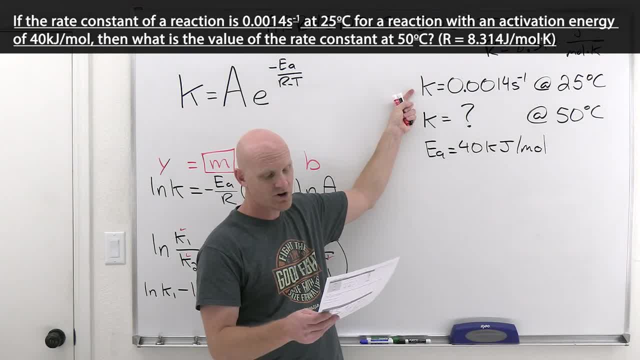 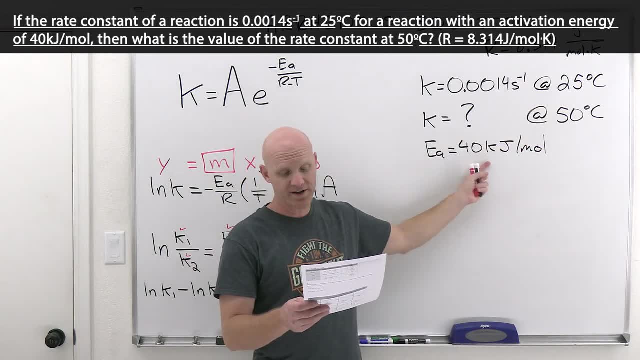 if the rate constant of a reaction is 0.0014 s to the minus 1, seconds to the minus 1, at 25 degrees Celsius for reaction with an activation energy of 40 kilojoules per mole, then what is the value of the rate constant at 50 degrees Celsius? 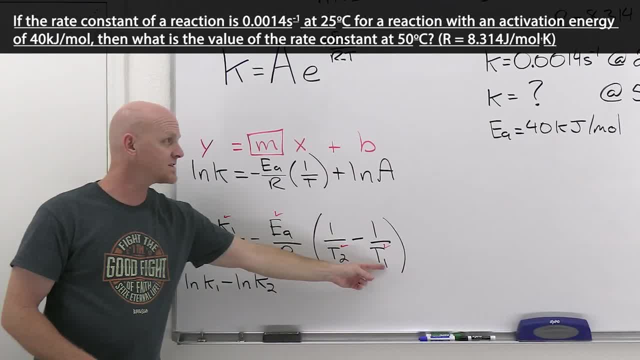 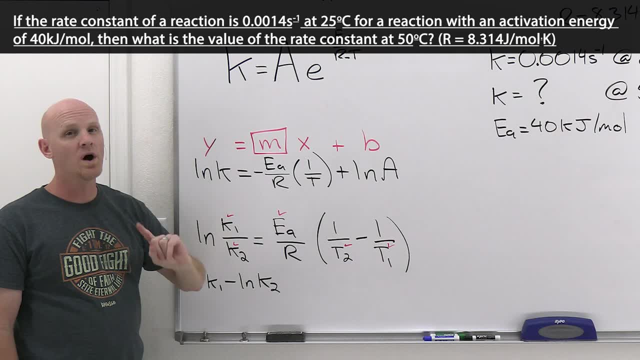 So in this case again, there are five variables in this equation K2.. We are given both of those. We're going to have to convert them to Kelvin, but we're provided with both of those. There's two rate constants and we're given one of those two. 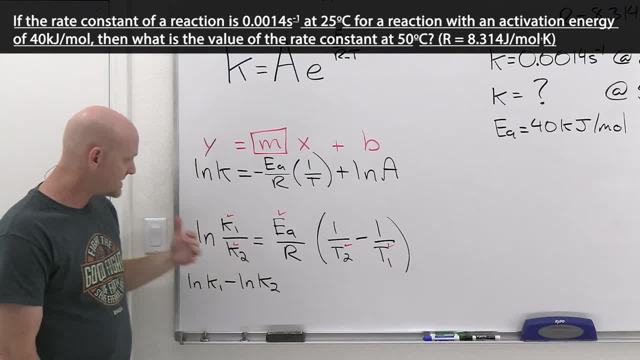 and then there's an activation energy and we're provided with that as well, And so in this case it turns out K1 and K2, it doesn't matter which is which It's not like. K2 has to be higher than. 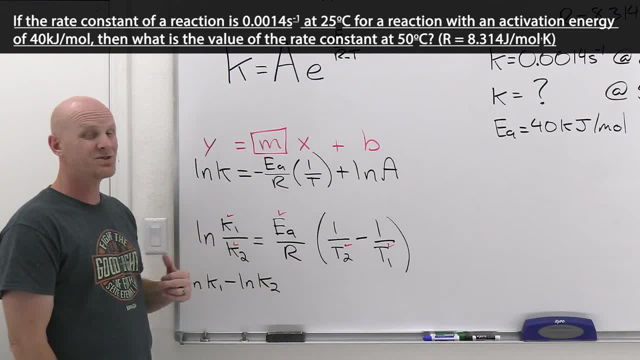 K1. It's actually arbitrary And so you can choose whichever. And if you're solving for K, this is the worst possible scenario, because you're going to solve for something under a natural log and that might involve a little algebra. that's a little fuzzy in your mind. 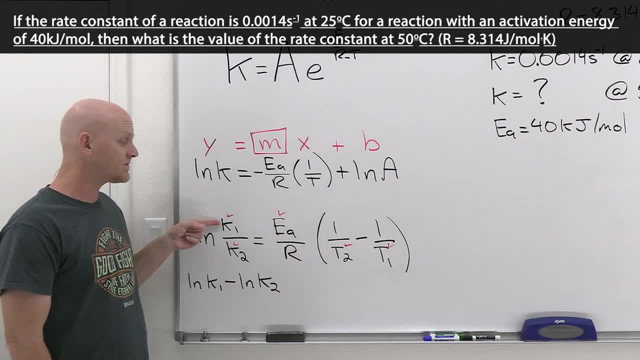 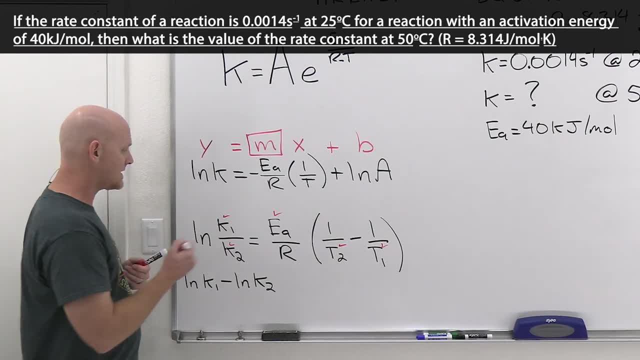 But in this case, if you've got the choice, though, it is going to be a little easier to solve for K1 in the numerator than it would be for K2 in the denominator, just purely from an algebra standpoint. And so I'm going to make K1 the rate constant at 50 degrees Celsius. 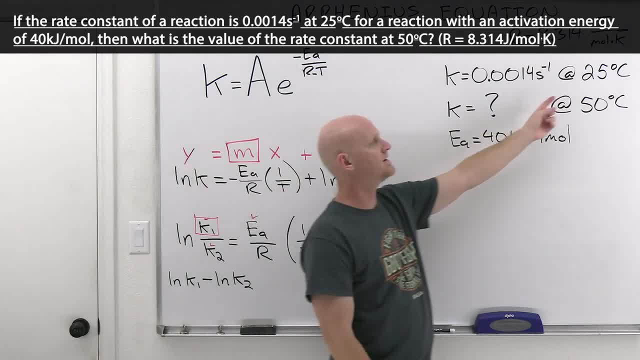 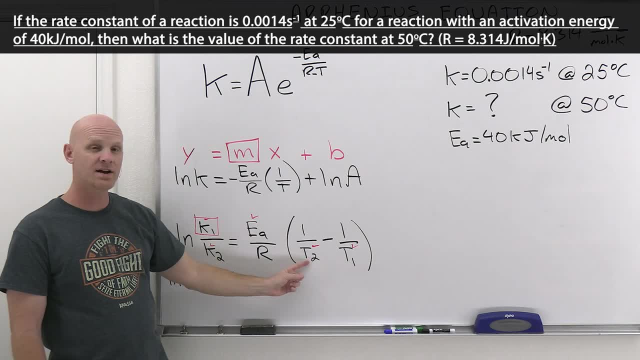 and I'm going to make K2 the rate constant at 25 degrees Celsius, And so I just have to be careful that if K2 is the rate constant at 25 degrees Celsius, then I have to make sure that I convert 25 degrees Celsius to 298 Kelvin and plug that in for K2.. So I'm going to make K1 the rate constant. at 50 degrees Celsius, and I'm going to make K2 the rate constant at 25 degrees Celsius, And so I just have to be careful that if K2 is the rate constant at 25 degrees Celsius, then I have to make sure that I convert 25 degrees. 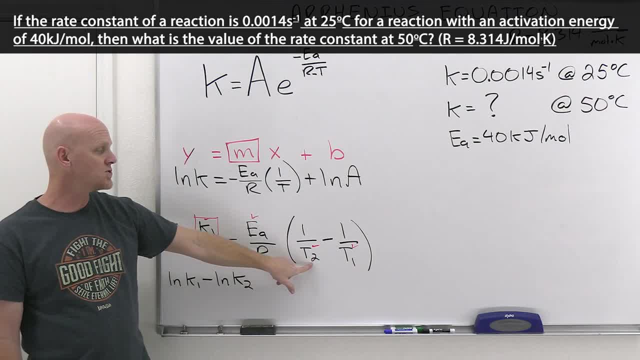 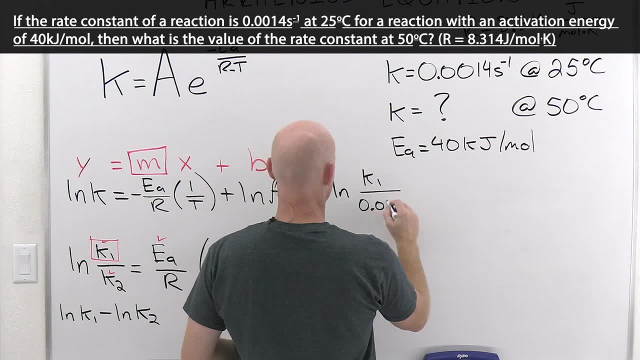 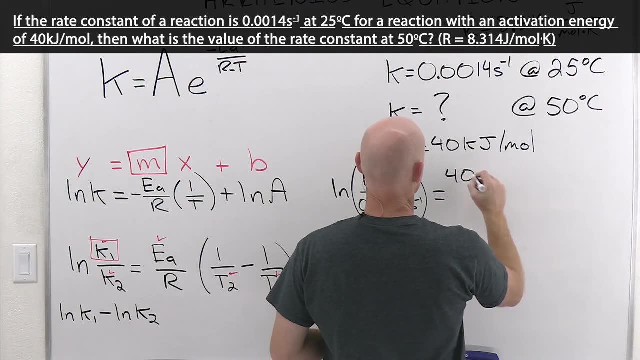 Celsius to 298 Kelvin and plug that in for T2 right here. Let's see how this works out. So ln of K1 all over 0.0014 S to the minus 1 equals Ea over R And in this case, 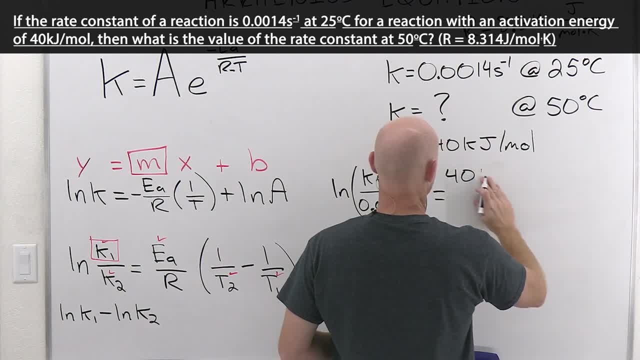 I've got 40 kilojoules- I'll write this a little different- Per mole, over 8.314 joules Per mole Kelvin, And we'll stop there for a second. This is again one of those commonplaces. 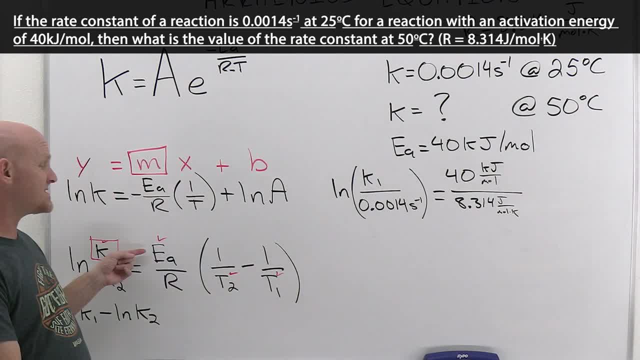 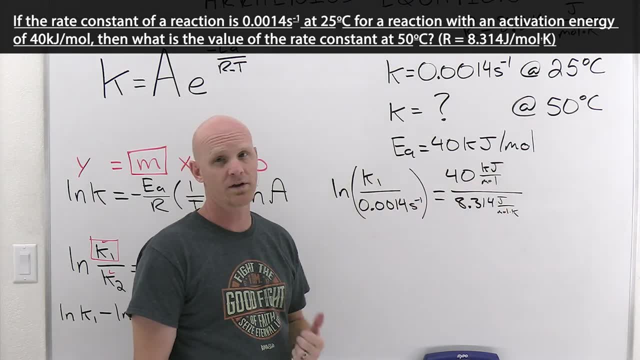 students make a mistake, because the activation energy, as it was supplied, was in kilojoules per mole. The R value is typically given to you is going to be in joules per mole Kelvin. These need to match. You need to convert one or the other And whether you want to convert 40 kilojoules per 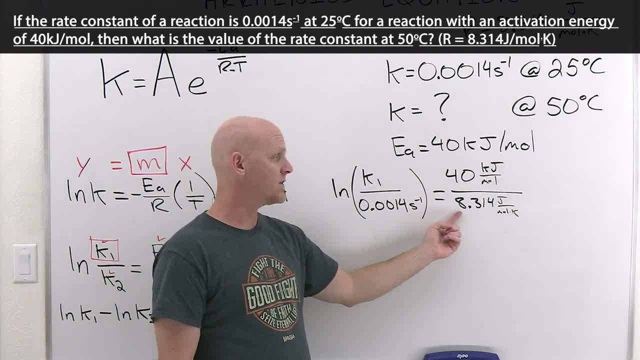 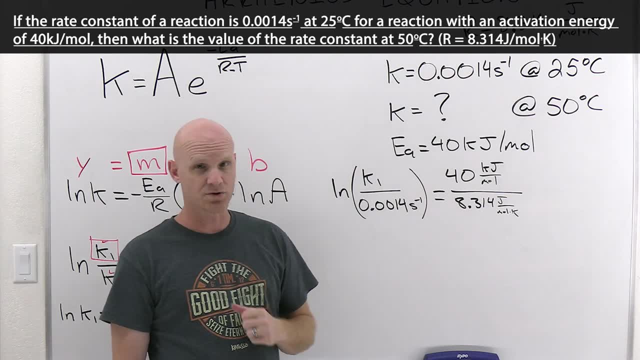 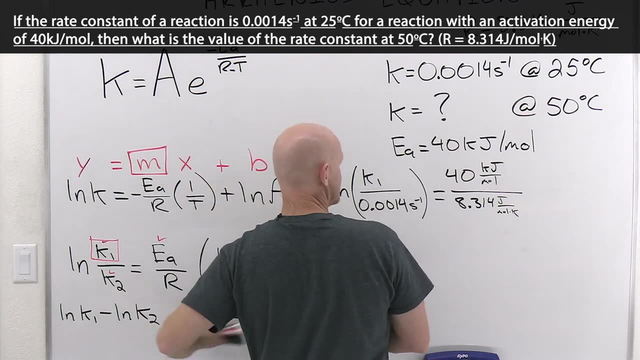 mole to 40,000 joules per mole, or if you want to convert 8.314 joules per mole Kelvin to 0.008314 kilojoules per mole Kelvin, it is your choice. My preference, though, is to convert 40 kilojoules to 40,000 joules instead, And that's what I'm. 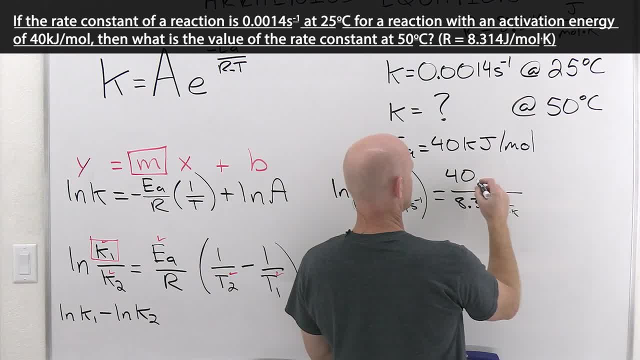 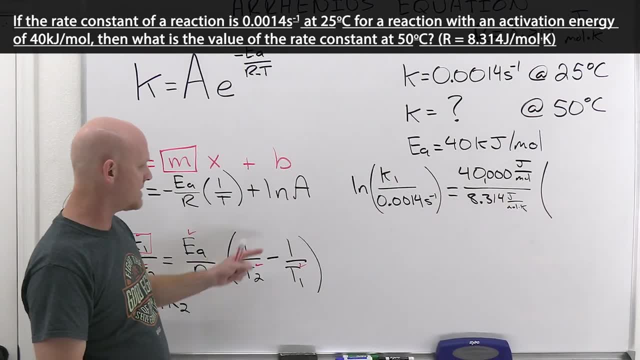 going to do here so that this works out properly. So we'll make this 40,000 joules per mole And then we've got 1 over T2 minus 1 over T1.. And again we said K1 was going to match up with. 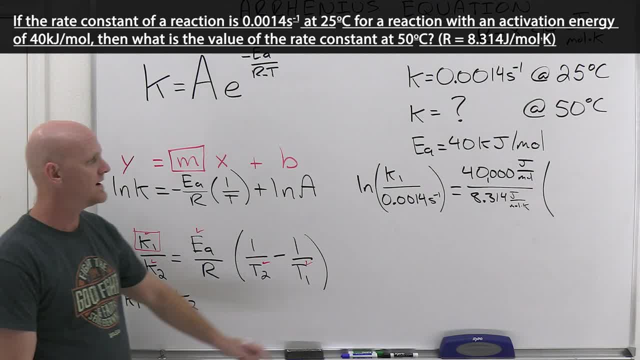 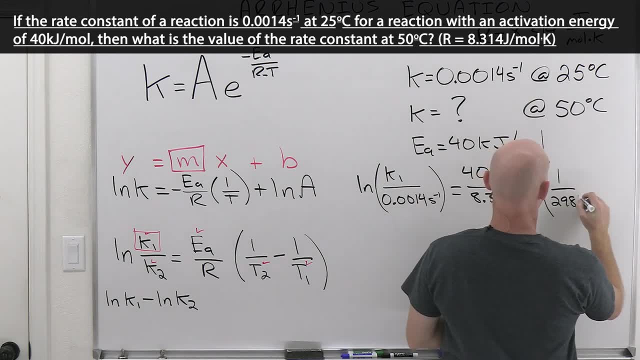 T1. And then K2 is going to match up with T2. And the K2 is the one I plugged in. that corresponds to 25 degrees Celsius, which corresponds to 298 Kelvin. Oh yeah, that's the right one. I almost got that backwards myself, So I told you. 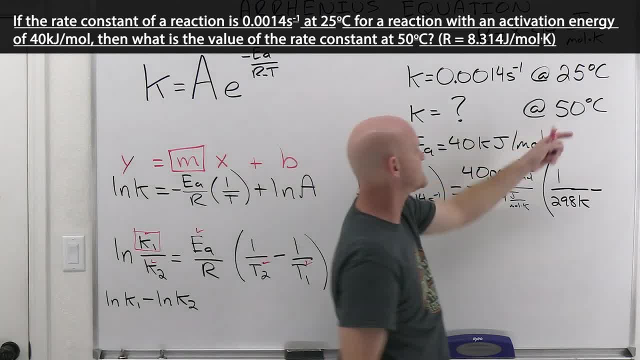 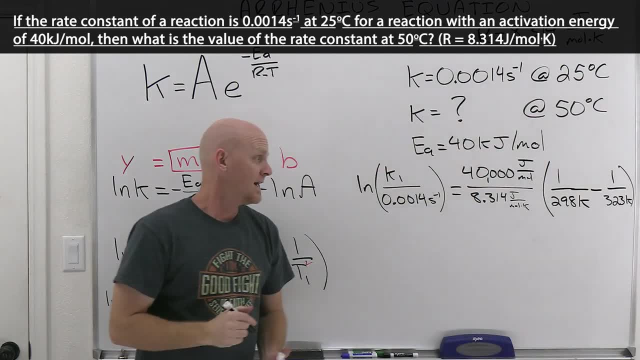 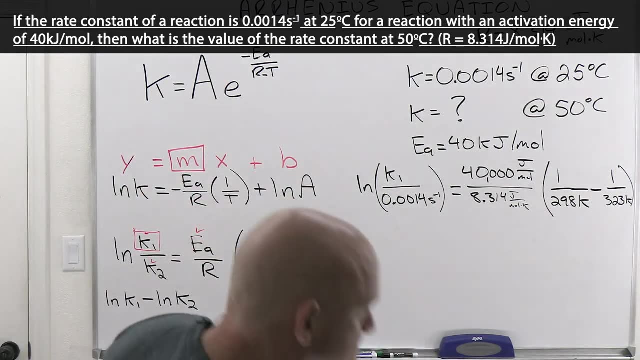 it's tricky. And then, finally, 1 over T1, well, in this case, 50 degrees Celsius is 323 Kelvin, And here we go. So let's pull out the calculators- and I have one here somewhere, All right. so first thing I'm going to do here is do 1 over 298 minus 1 over 323.. 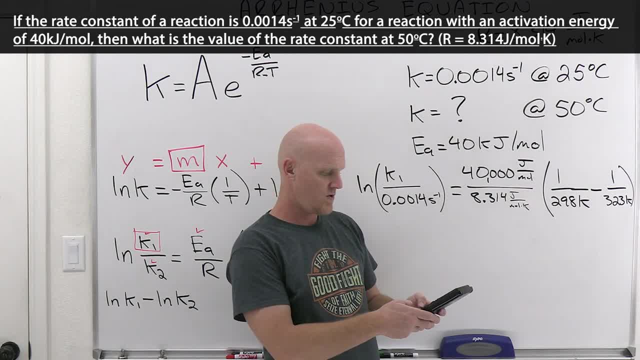 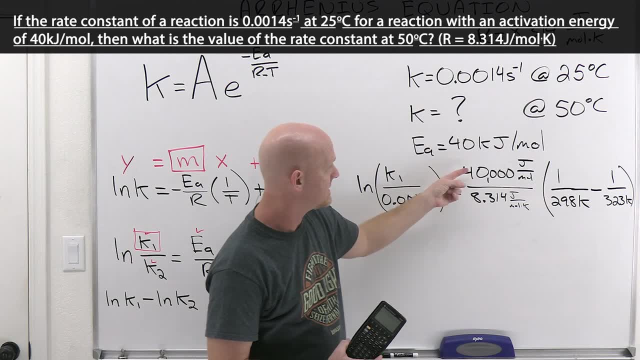 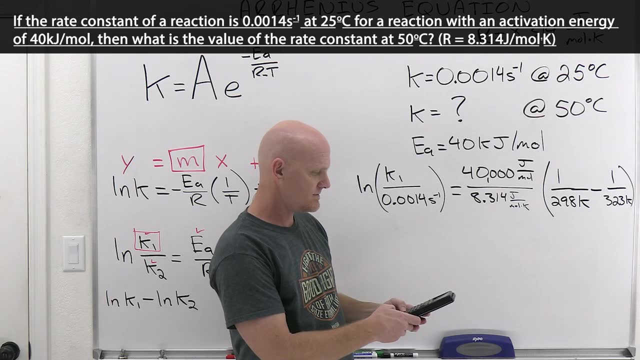 So 1 divided by 298, minus 1 divided by 323.. And then I'm going to get an answer, but I'm not going to stop there. I'm going to then multiply this by this ratio, So times 40,000 and divided by 8.314.. 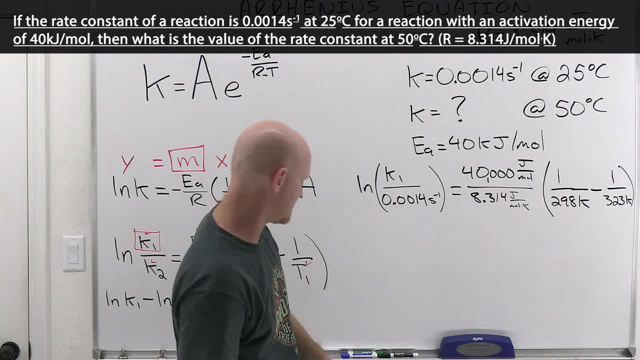 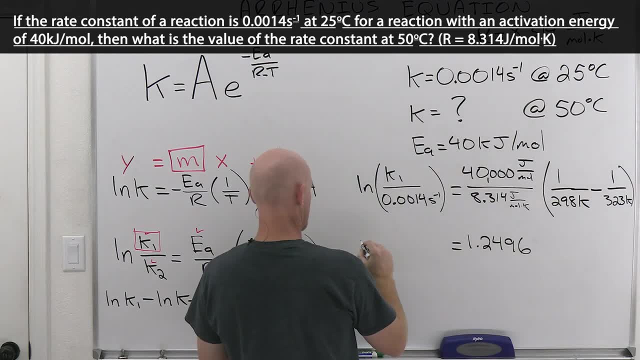 And now I'm going to stop there, and that's 1.2496.. And that's what the ln of k1 over 0.0014 is going to equal. Okay, so now we've got to solve for something that is under the natural log. 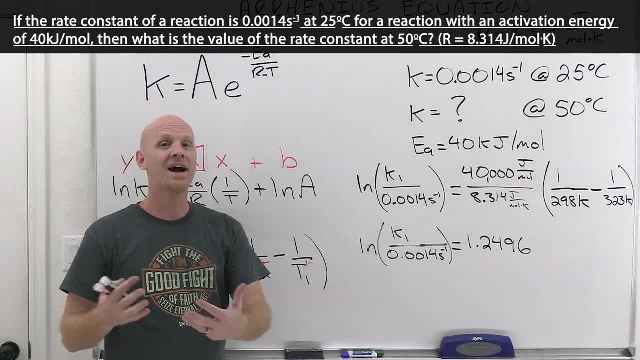 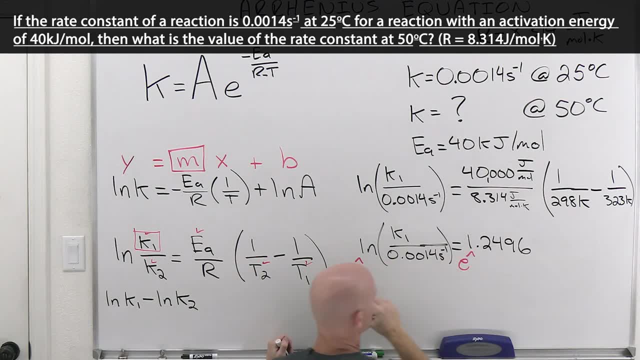 And so we've got to get rid of that natural log. And the way we get rid of that is by remembering that the exponential was the inverse function here, And so we're going to take e to this power here and e to this power here, on both sides. 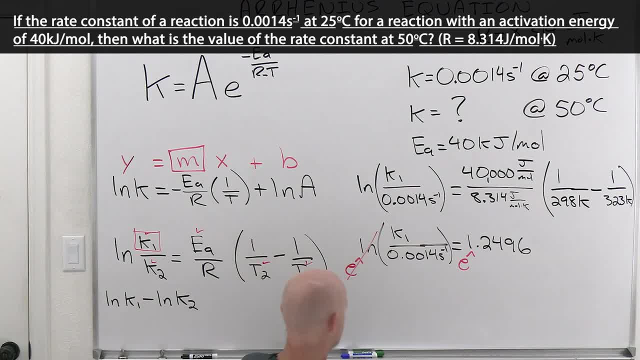 But here it's going to cancel And so we're going to be left with k1. over 0.0014 equals e to the 1.2496.. And I'm going to work that out. So in this case, e to that last answer in my calculator is 3.49.. 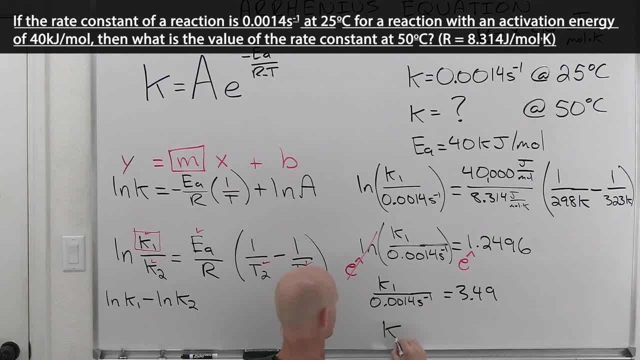 Cool, and then I'll just multiply that up by the 0.0014.. 0.0014., 0.0014., 0.0014., 0.0014., 0.0014. And we're going to get k1 equal to 0.00488.. 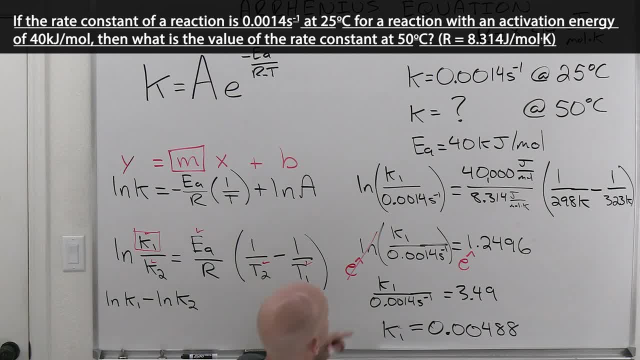 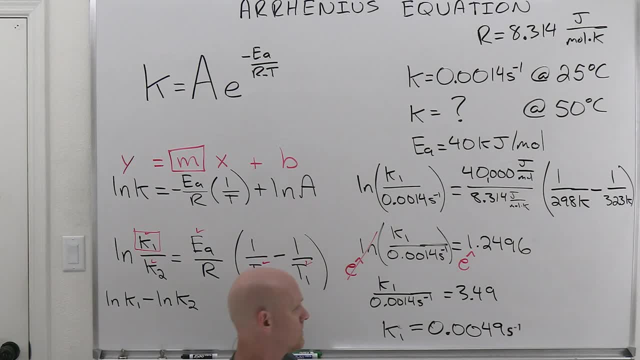 I probably actually should only give this in 2 sig figs, since the original one was only given in 2 sig figs, So we'll round this to 0.0049.. Cool, so, by going from 25 degrees Celsius to 50 degrees Celsius. 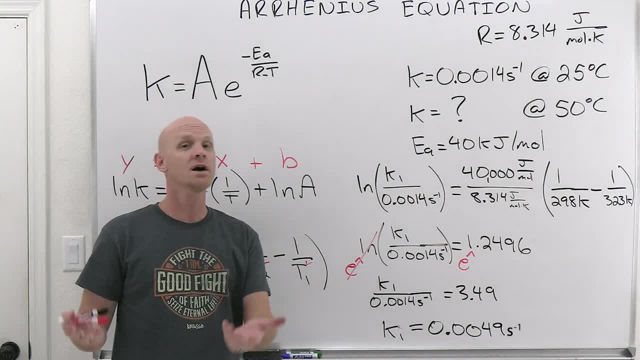 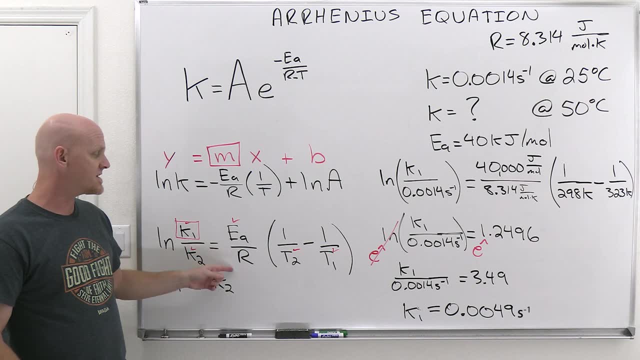 an increase in temperature. yes, the k value got bigger And in this case roughly 3.5 times bigger. So once again, lots of places you can go askew on this one. Make sure your temperatures are in Kelvin. Make sure activation energy and R are in the same units. 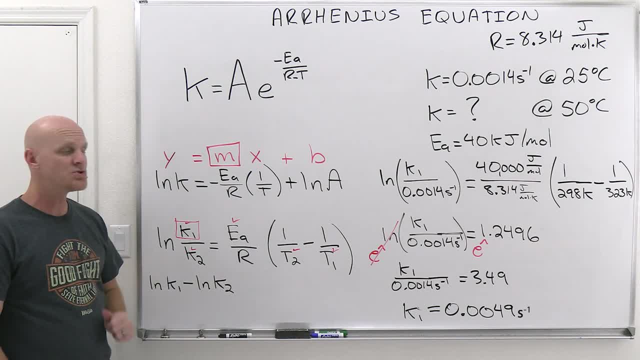 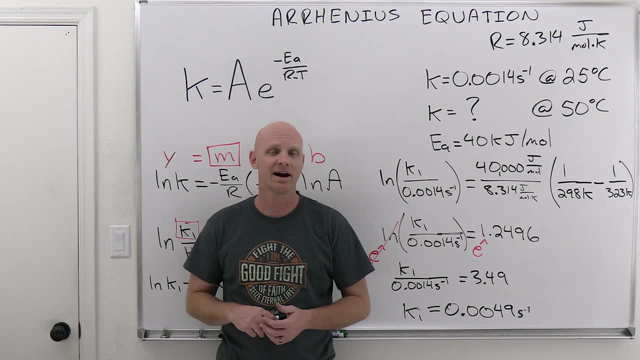 And then if you're solving for something under the log, you've got to remember that it's the exponential that's going to allow you to do that. Now, if you found this lesson helpful, then smile at a random stranger and have a great day.